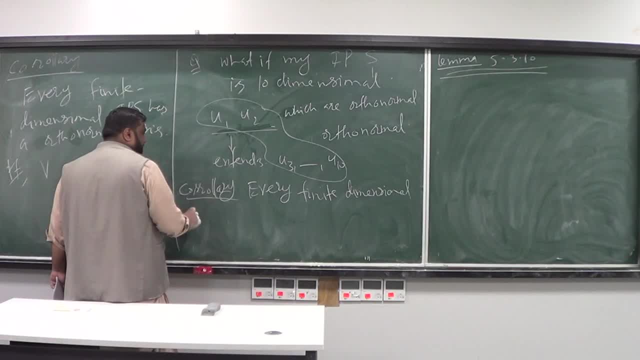 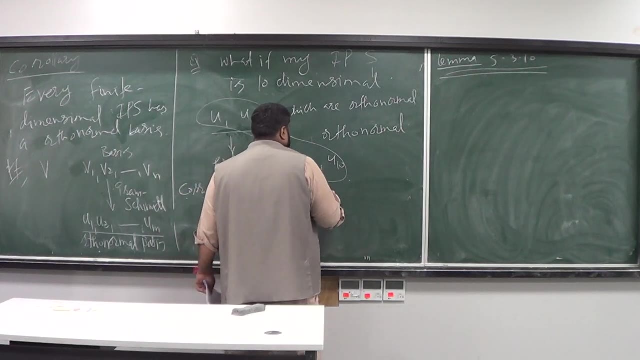 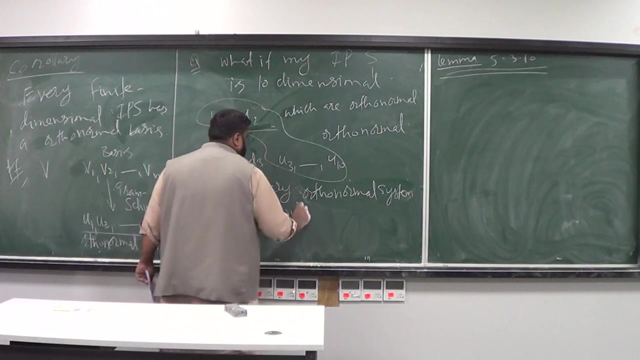 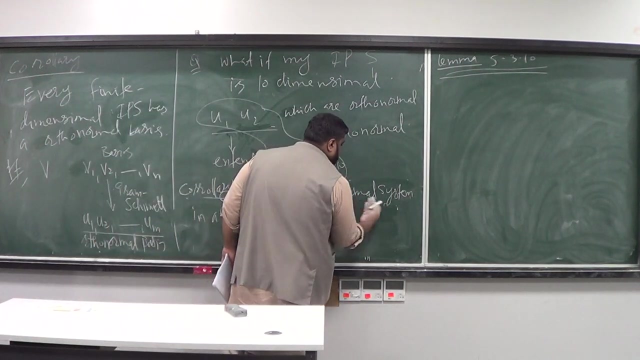 in a set of orthonormal vectors, every, every finite dimensional, every orthonormal system. imagine: you have an orthonormal system in a finite dimensional vector space. you can extend this orthonormal system in a finite dimensional vector space or vector space, again and again. 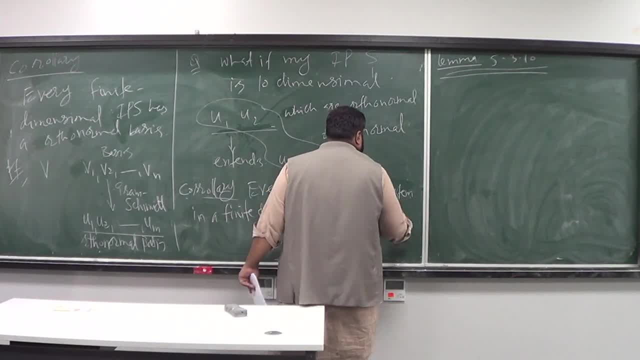 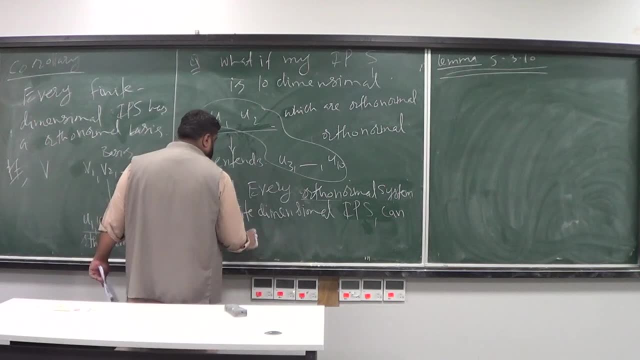 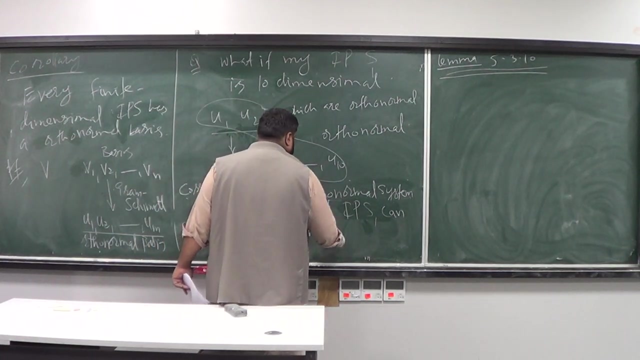 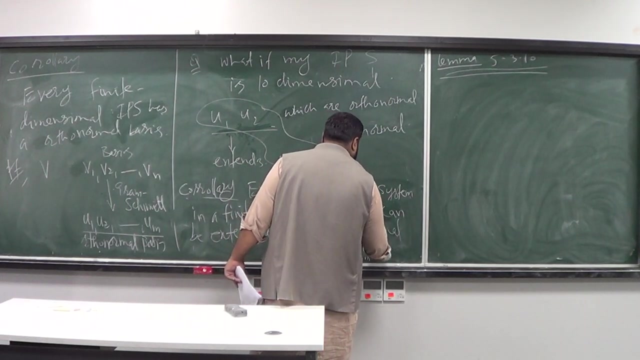 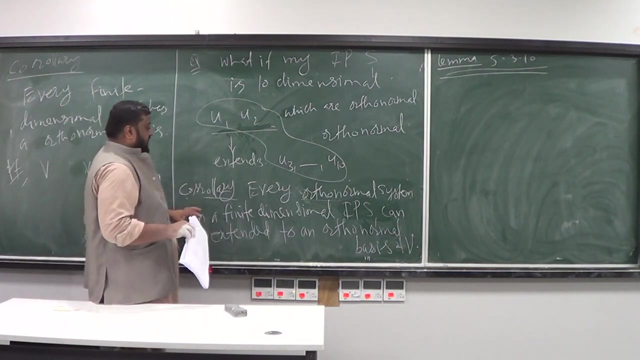 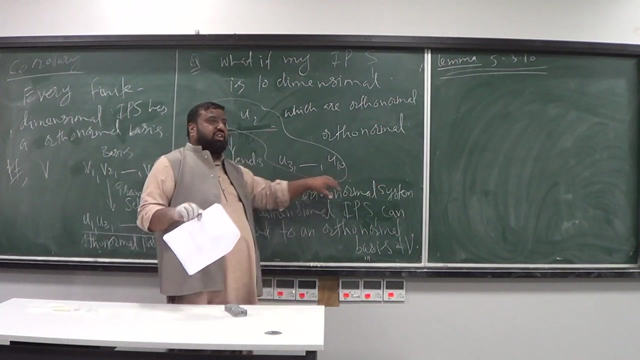 in a product space can be extended, can be extended to an orthonormal basis, orthonormal basis of it. ok, here is the thing: you have a finite dimensional in a product space and you have some orthonormal vectors. then you can take some orthonormal vectors. 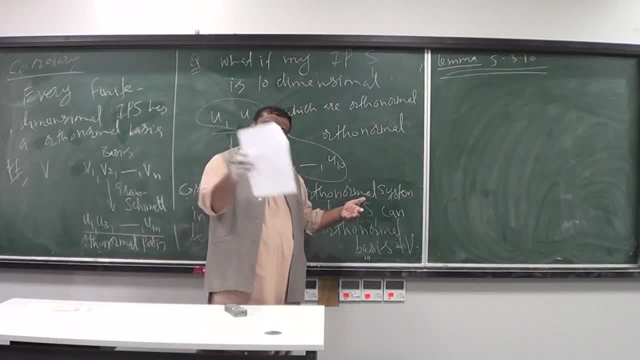 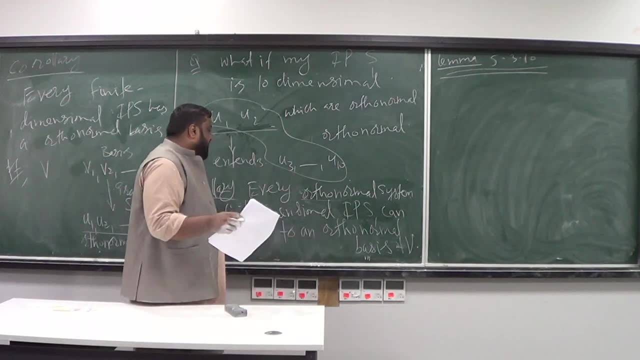 and extend them. in other words, you can add some more orthonormal vectors to them, ok, which are unknown, and turn them into an orthonormal basis of V, actually, ok, in the orthonormal basis of V. so how you gonna do it? how you gonna do it? 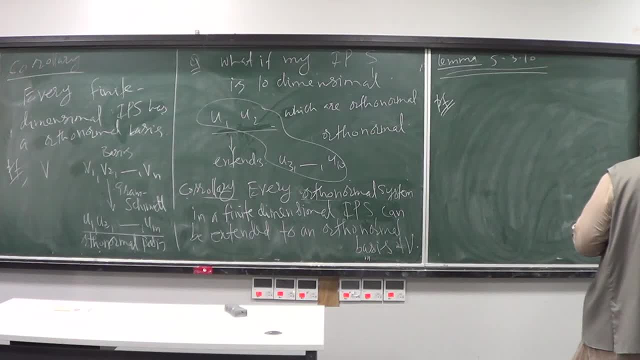 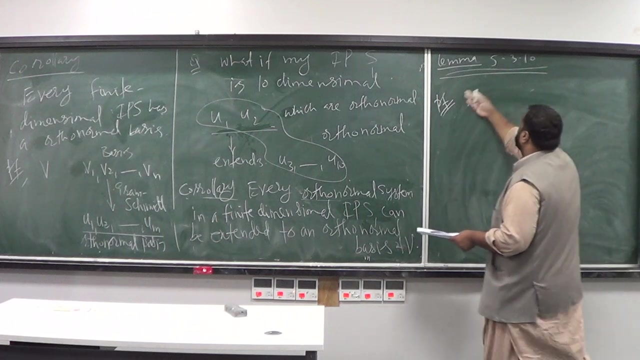 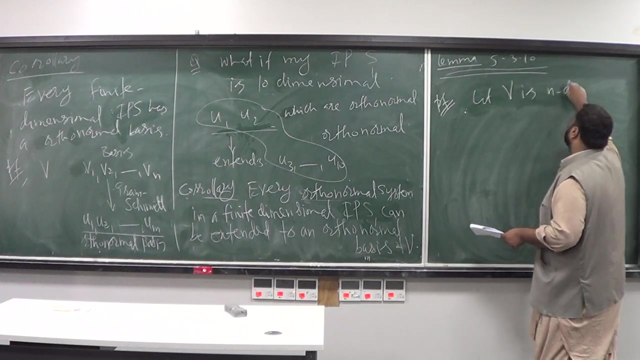 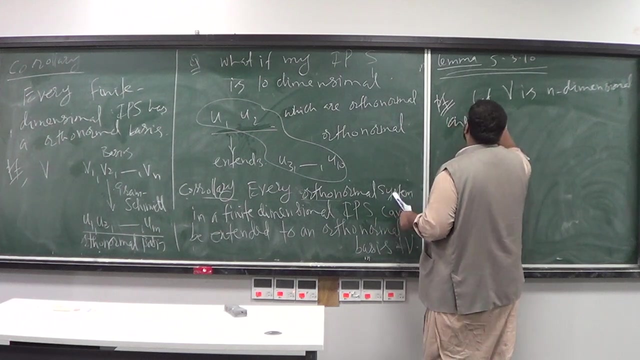 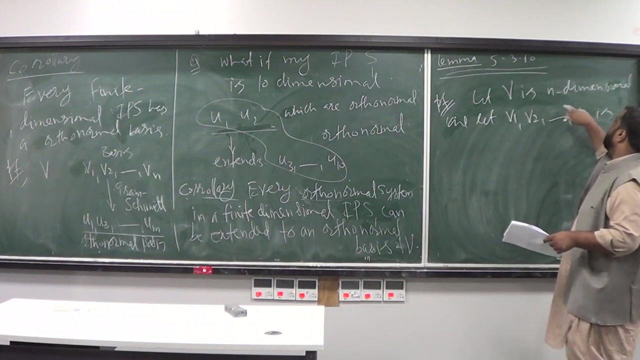 how you gonna do it. so imagine, imagine you have been given an orthonormal system. given, imagine, let let V vector space V in a product space V is n dimensional. ok, is n dimensional. lets assume that. and and let V1, V2, Vr, where r is some number that is smaller than n. 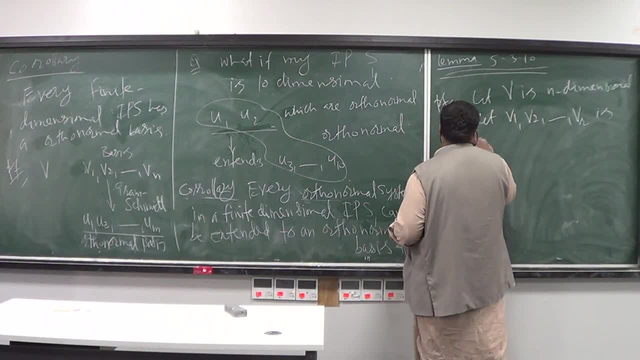 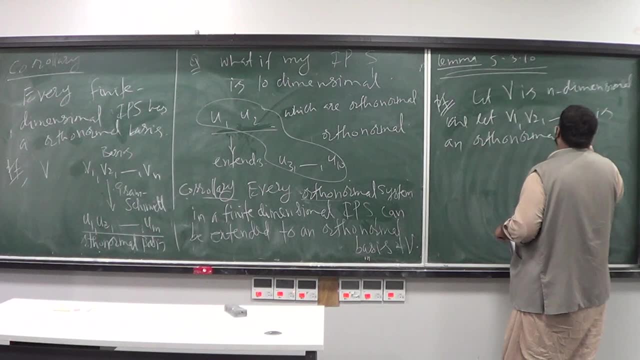 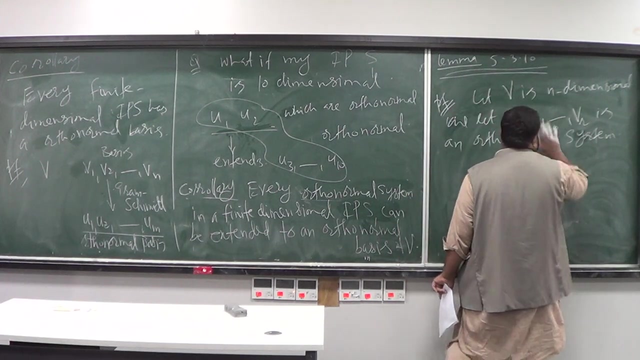 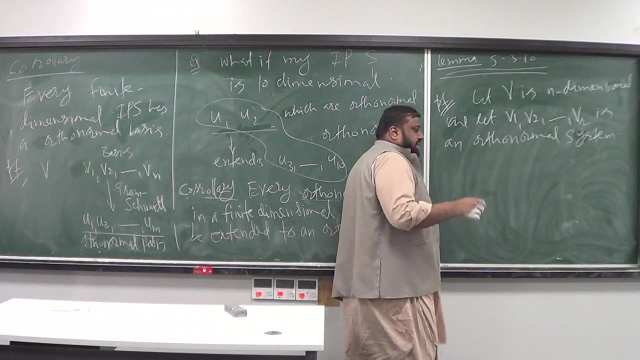 is an orthonormal system. is an orthonormal system, ok then. then what is an orthonormal system? question, can I extend this to the orthonormal basis? the answer is yes, why? because from your first linear algebra course you know very well: 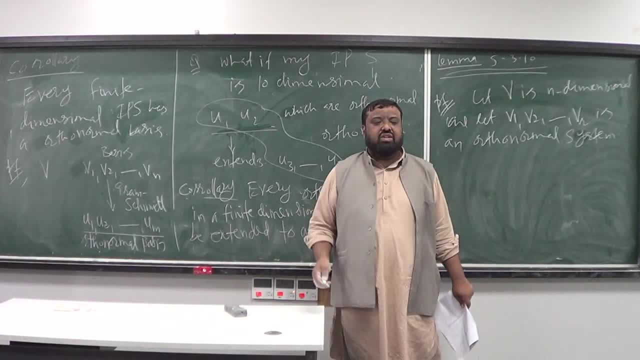 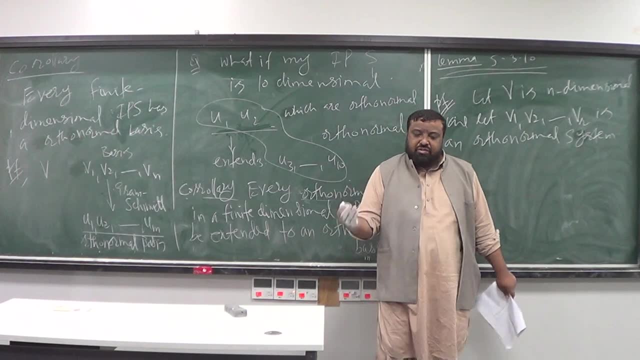 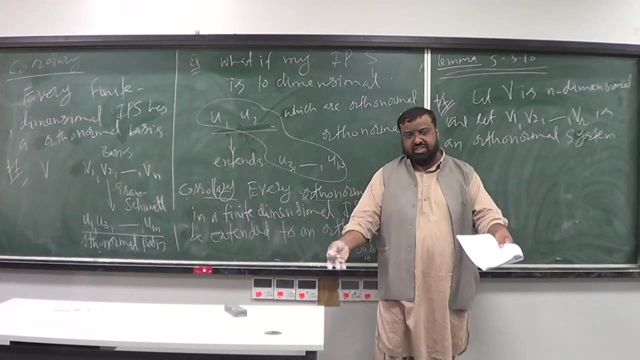 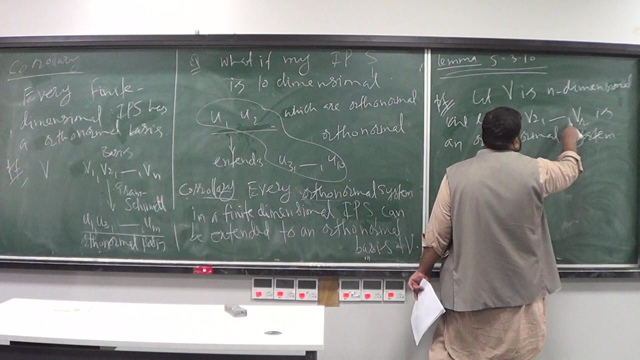 that if you have, for example, a five dimensional vector space in which you have three vectors that are linearly independent, ok, then you can find two more vectors and put them together. that can form basis for what do you call the vector space. so so lets take V1, V2, Vr. 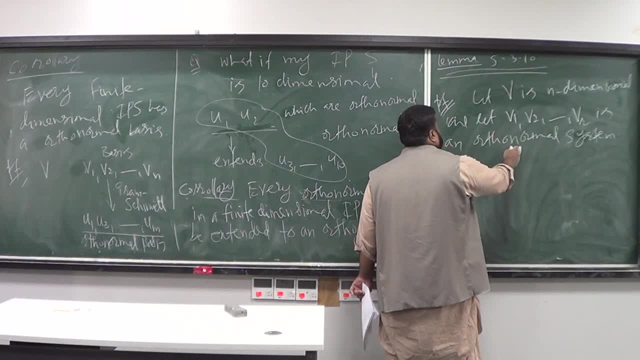 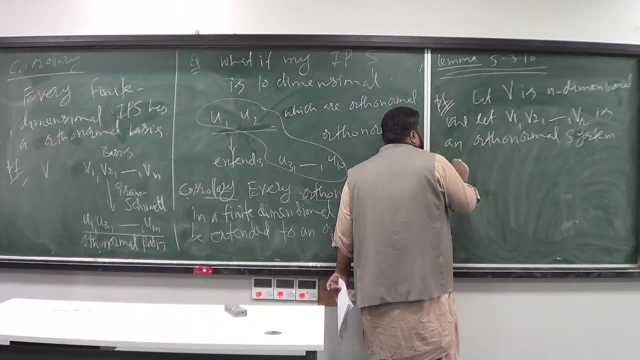 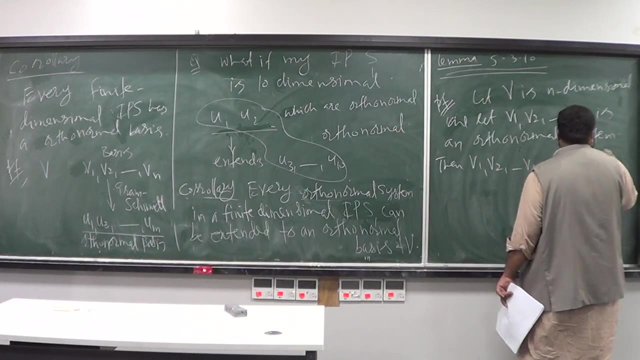 they are not only orthonormal vectors, but they are vectors in the inner product space, V. and then this V1, V2, Vr can be extended, can be can be extended to a basis. ok, so now we are going to get into the details of it. that. 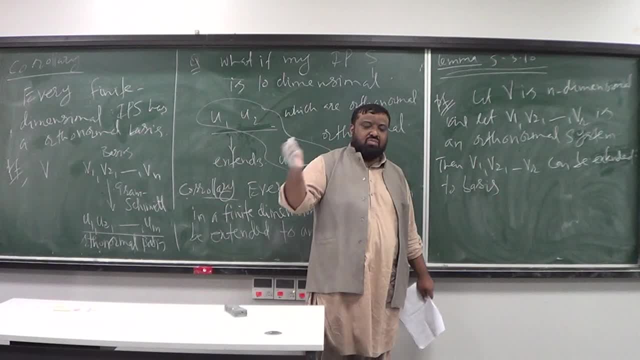 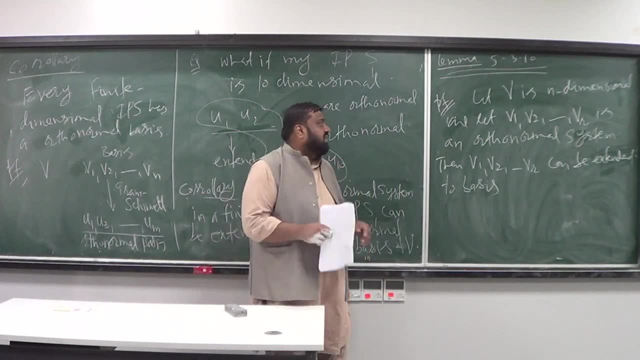 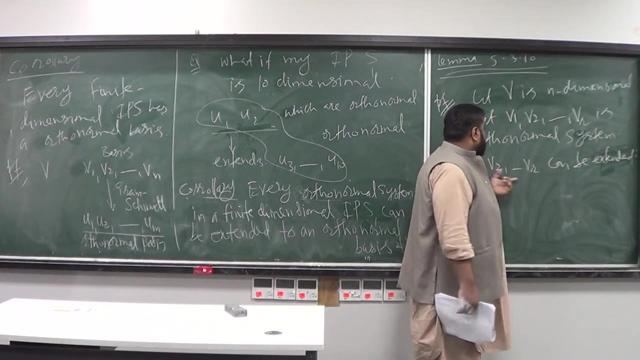 how to add some more vectors in a given set of vectors to form what do you call a basis. actually, so same thing. so another thing that is obvious is that since this is an orthonormal system, so all of these vectors must be linearly independent. so what we can do in these linearly independent vectors, 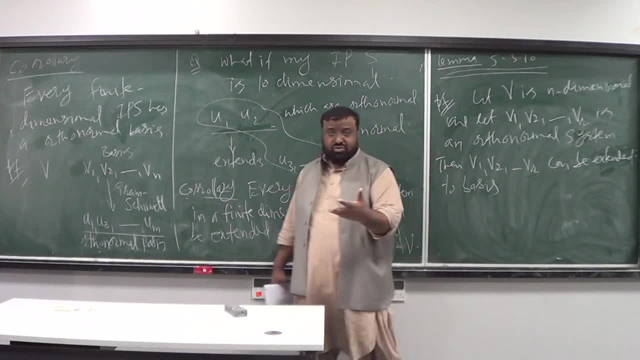 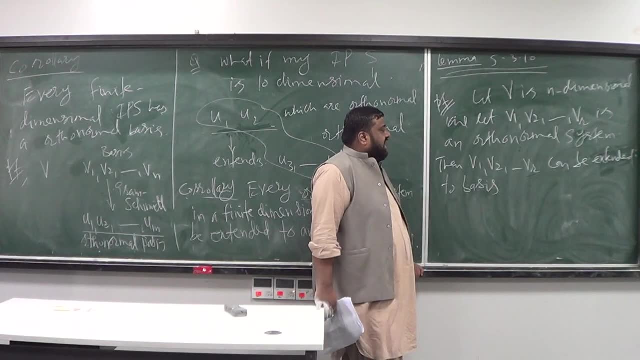 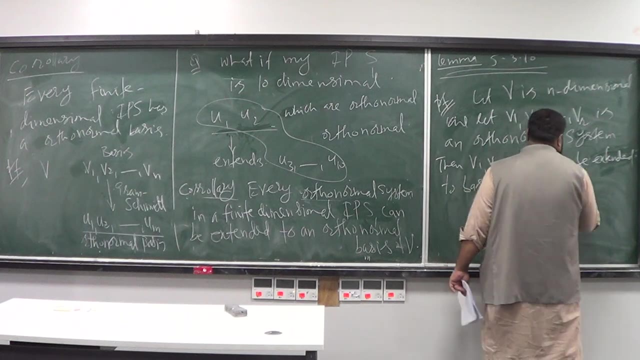 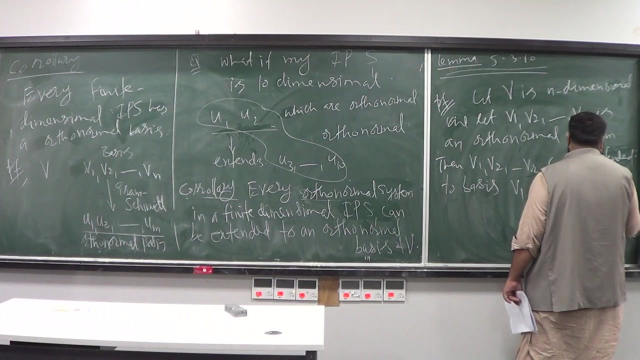 from the linear algebra that you learnt in your first course what we can do. you can extend this. what do you call basis? extend these r vectors to a basis that comprises of m vectors, into V2, V2, you know Vr, Vr plus 1 and up to Vn. 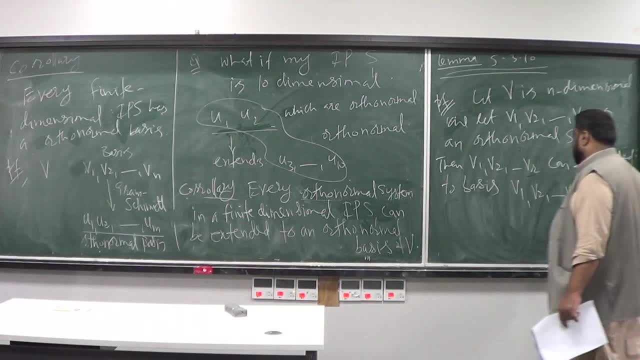 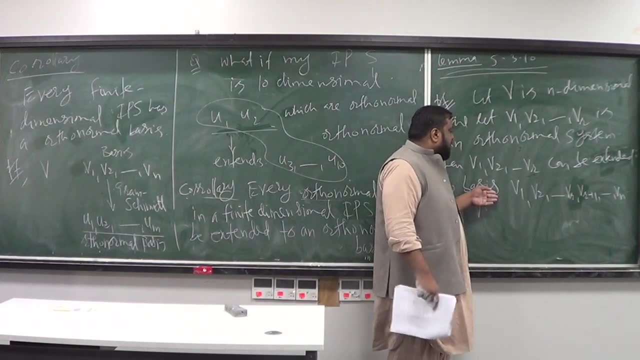 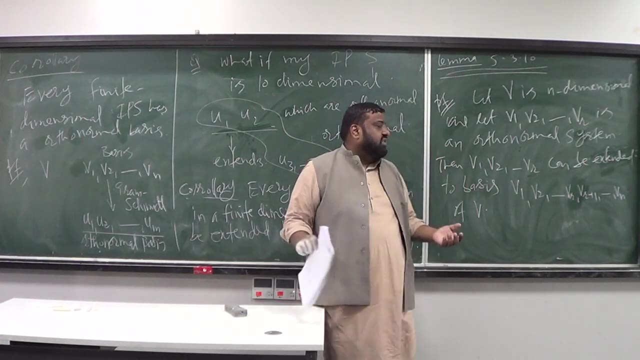 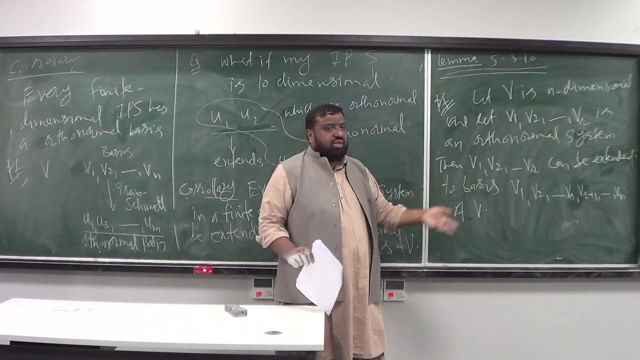 so you can do it. of V question: is it necessary that all of these vectors are this n vectors that you have extended? ok, are r vectors that you have extended and formed a basis for V is also an orthonormal system? the answer: there are two possibilities. 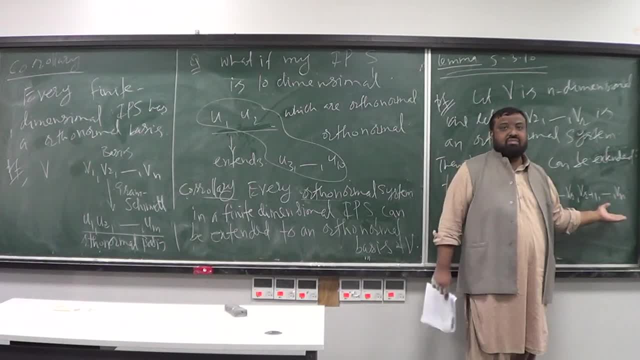 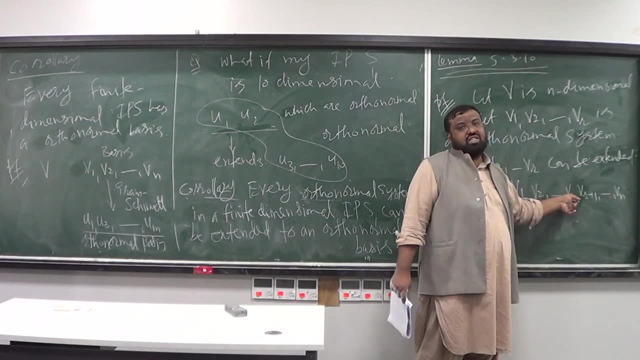 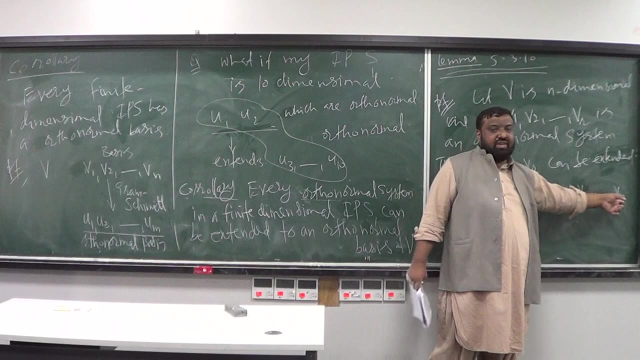 either this is going to be an orthonormal system. so if it is an orthonormal system, in other words V1 to Vr- I already know that it is orthonormal system and I added some more vectors to it. now there are two possibilities for all these n vectors. 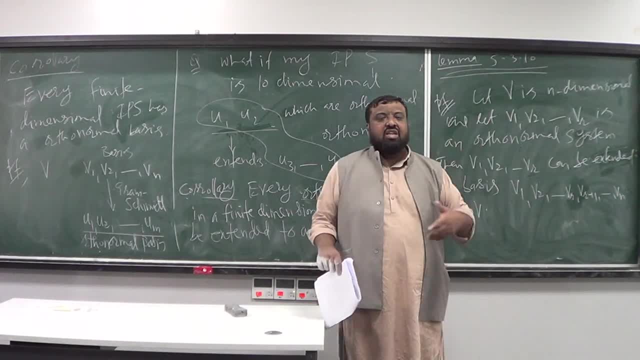 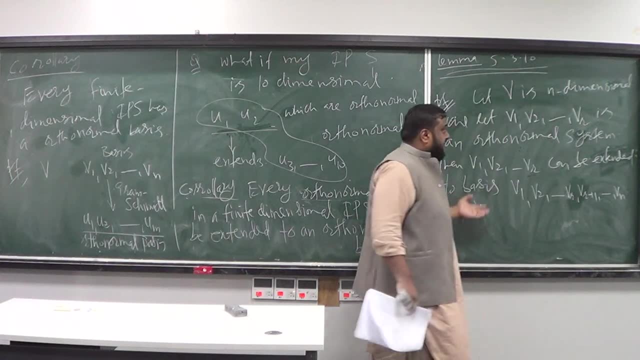 that either it is going to be an orthonormal system or if it is an orthonormal system. if it is an orthonormal system, this is then. this is already orthonormal basis actually that we want, but the other possibilities could be that ok. 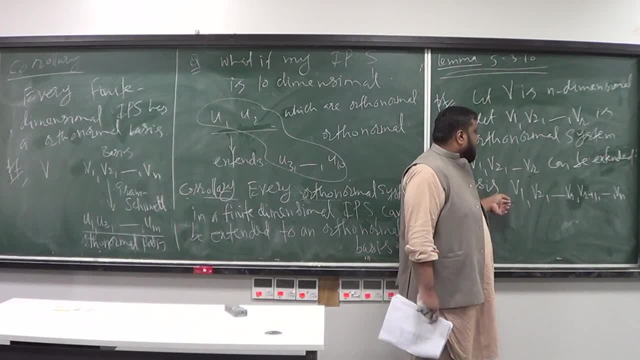 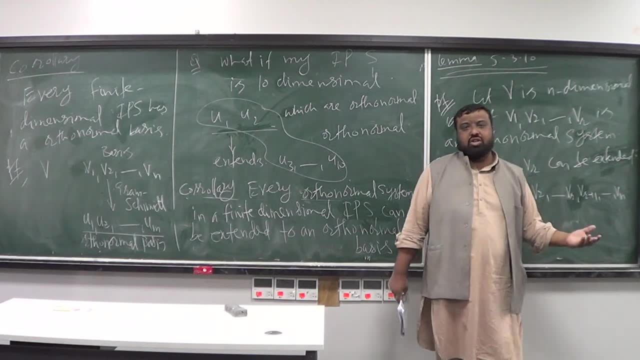 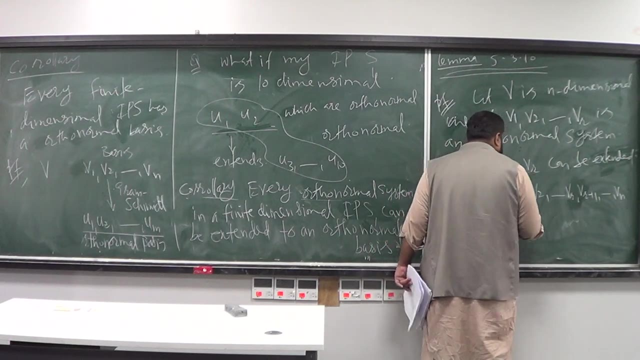 I know that V1 to Vr are orthonormal, but you know, this entire system, this entire set of n vectors does not forms an orthonormal system. so what you can do, you can take this system and apply what do you call a Gram-Schmidt. 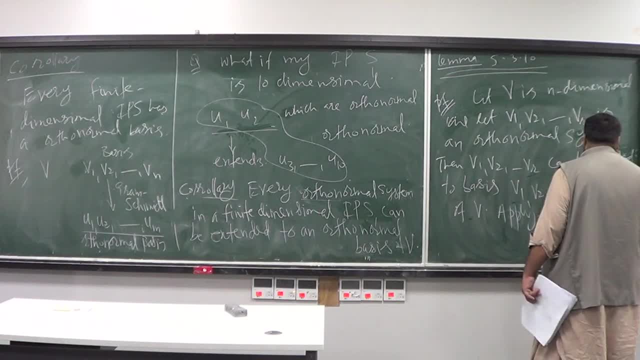 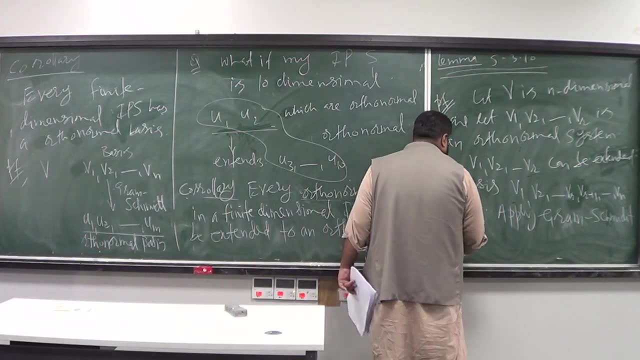 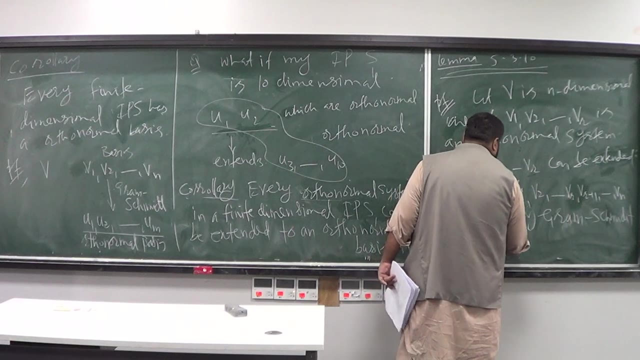 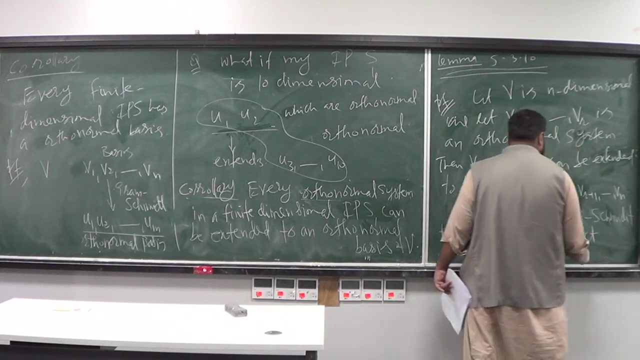 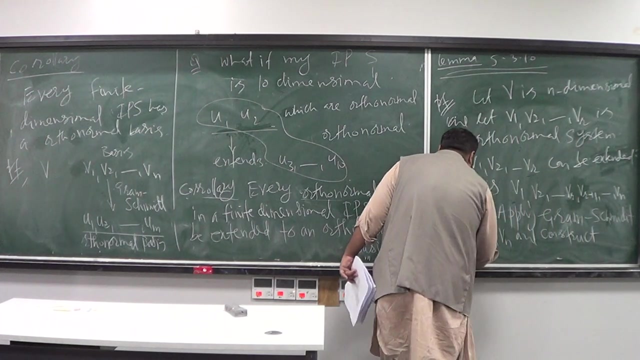 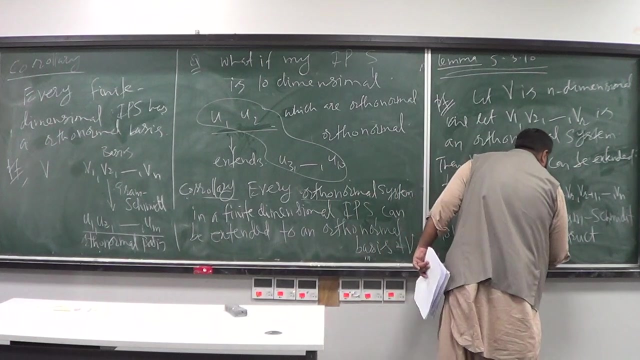 what do you call Gram-Schmidt? ok, and create an orthonormal system to V1, V2, Vn, and and construct. construct an orthonormal basis or orthonormal, yes, orthonormal basis, say U1, U2, up to Un, actually for V. 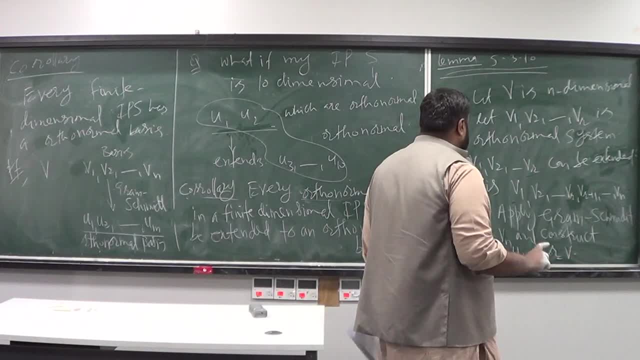 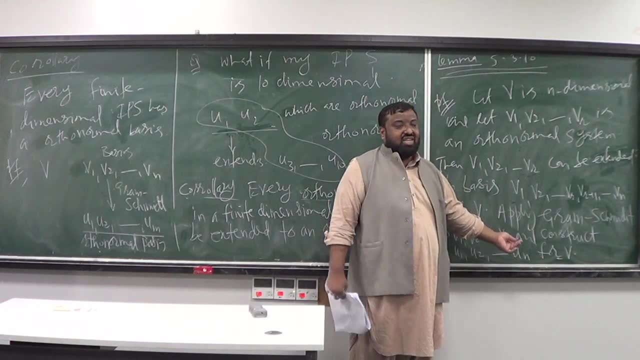 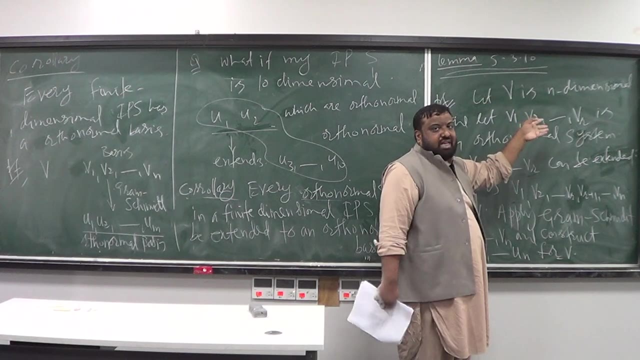 ok, but here is one little glitch. I wanted to extend this system. these might be the new vectors. actually, I don't want a new basis, an orthonormal basis for what do you call in a product space. I want to extend these vectors, in other words, in this list. 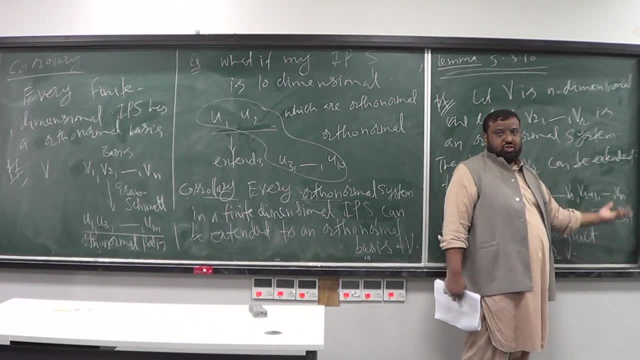 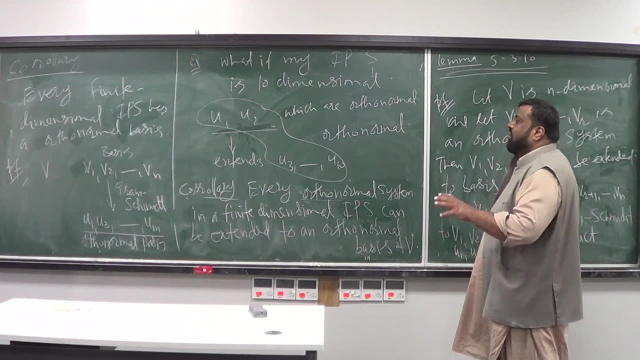 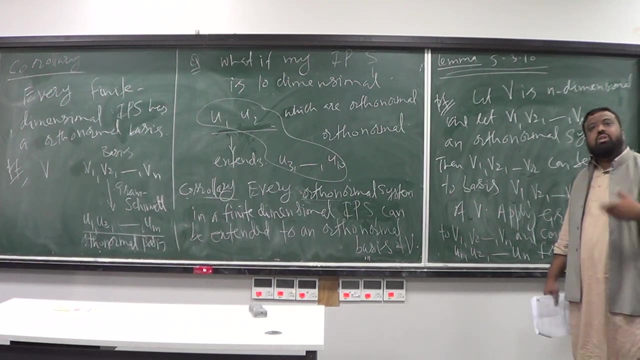 I want to add some more vectors that are orthonormal. but we just discussed actually that if your vectors are already orthonormal and you apply Gram-Schmidt on it on them, there will be no difference actually on them, so nothing will change in them. 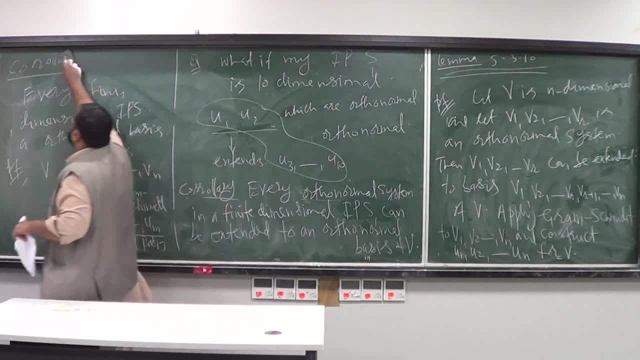 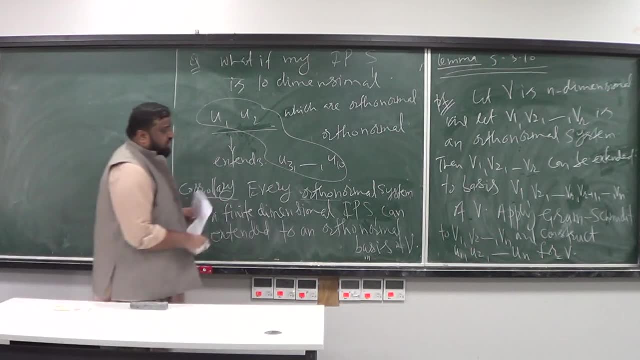 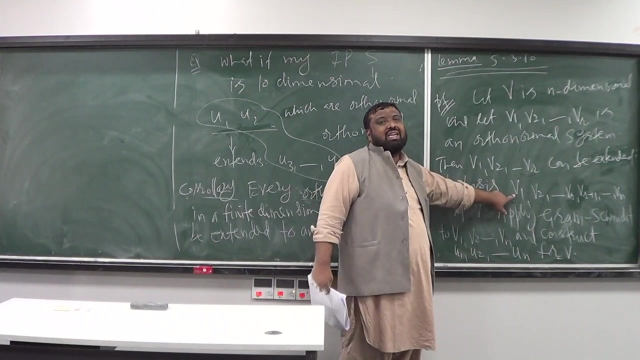 so, in other words, if you take Gram-Schmidt process and apply Gram-Schmidt process on what do you call V1, the Gram-Schmidt process will give you the same and obviously I can take what do you call the vector V1 and by applying the Gram-Schmidt process, 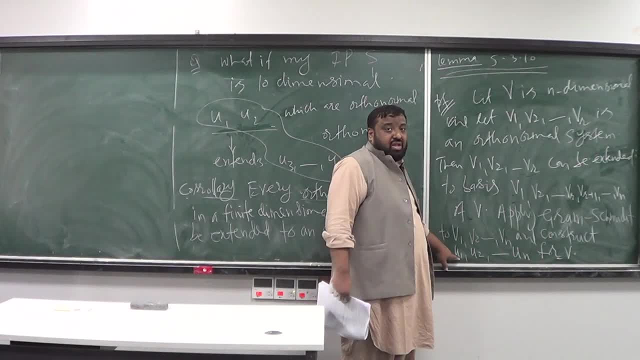 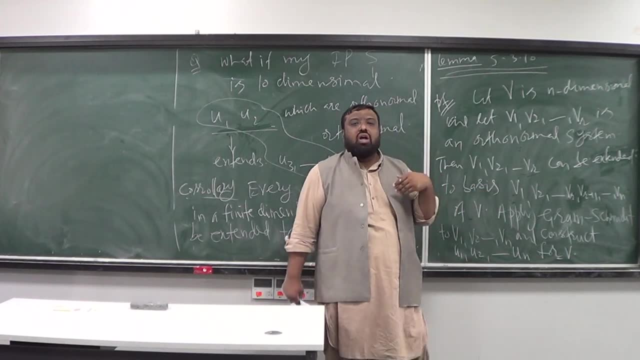 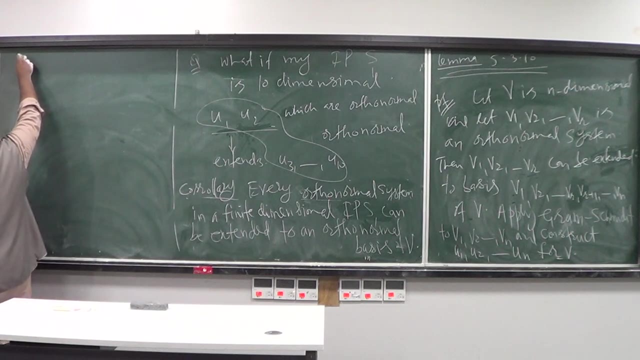 I can, I am going to get what do you call U1? but since you know, V1, V2, Vr is a part of what do you call an orthonormal system, so this U1 is not V1, is not going to change. in other words, this U1. 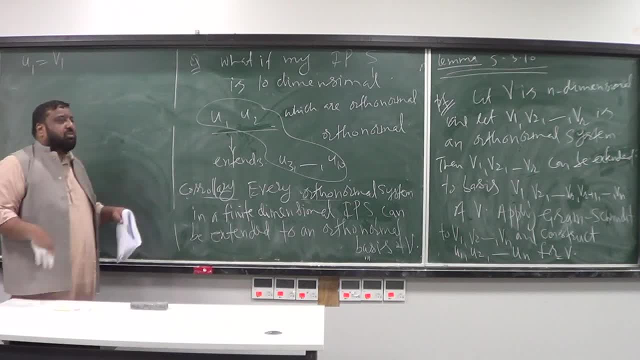 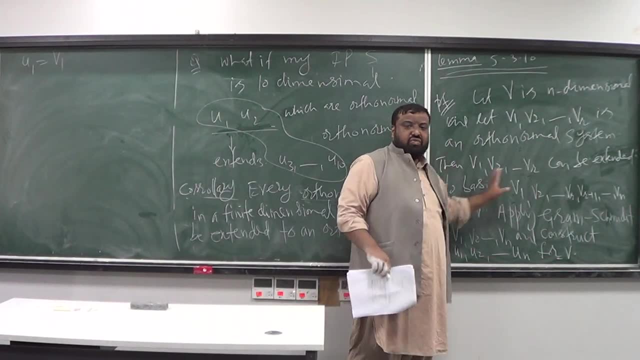 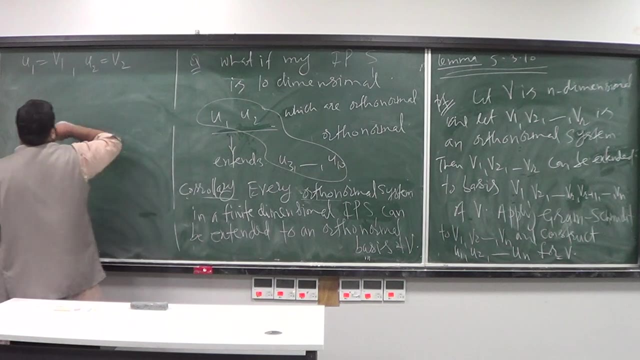 is going to be the same V1. in other words, the Gram-Schmidt process is not going to change these vectors V1 to Vr, so the V1 to Vr would stay same. in other words, your U1 is going to be same, your U2 is going to be same as V2. 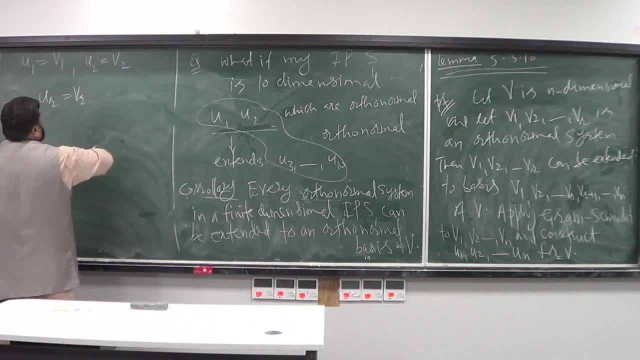 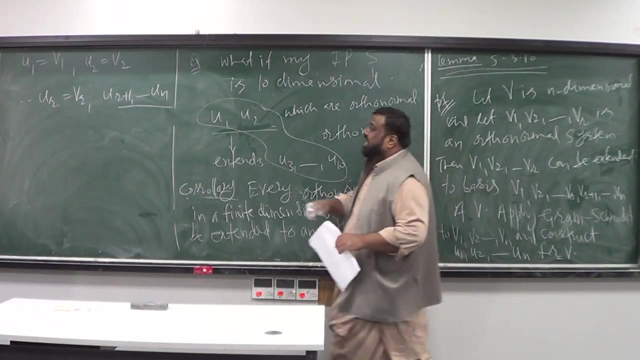 and up to your Ur is going to be Vr ok, and hence the new vectors: Ur plus 1 up to Un. these will be may be different from what do you call Vr plus 1 up to Vn, but the first R vectors under the Gram-Schmidt process. 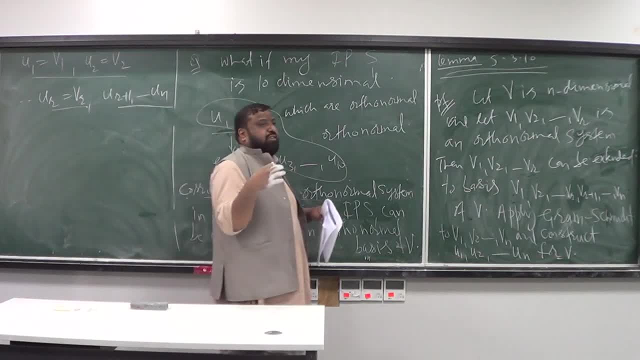 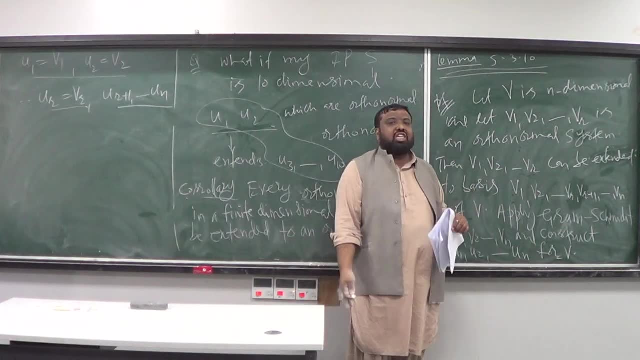 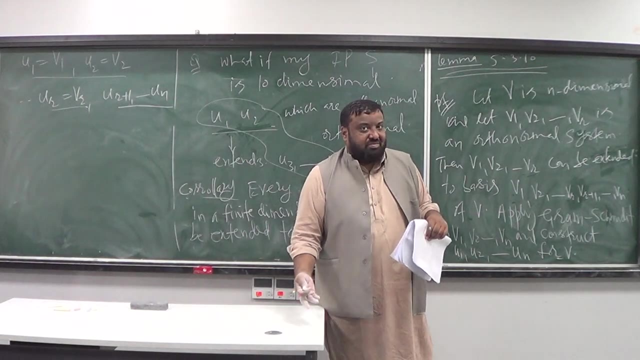 are going to stay same, because we know that. for when you apply the Gram-Schmidt process on an orthonormal set of vector, it does not change. it just returns the same vectors because the orthonormal vectors are already orthonormal. so the Gram-Schmidt process is not going to do anything. 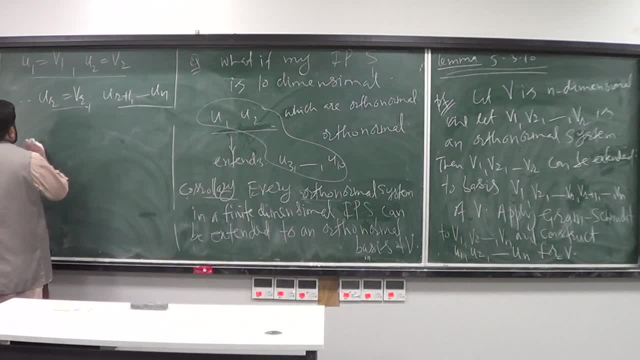 hence, what happens is that your new basis, new orthonormal basis that you have found- U1,, U2, Un- is basically this: V1, V2 up to Vr and Ur plus 1 up to Un. so, in other words, I took my orthonormal system. 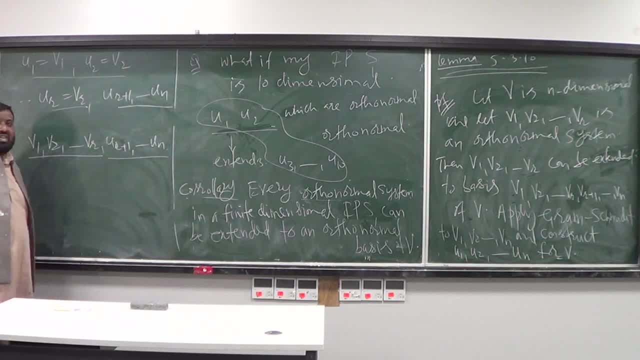 and I added some more vectors to it and I found- and I found an orthonormal system that is also a basis for the inner product space and hence this: this basis is orthonormal basis, vector, orthonormal basis. ok, I know in this first part of discussion, 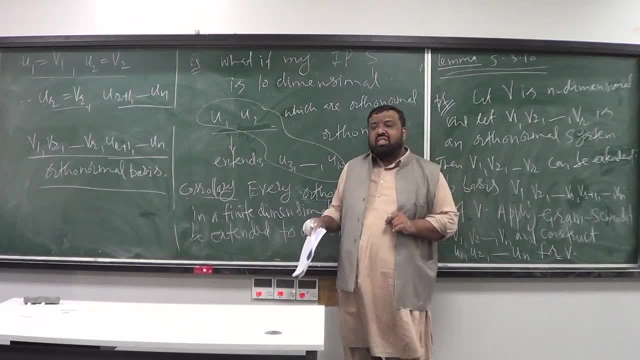 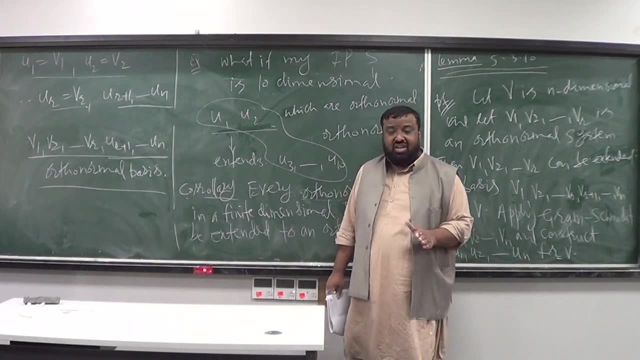 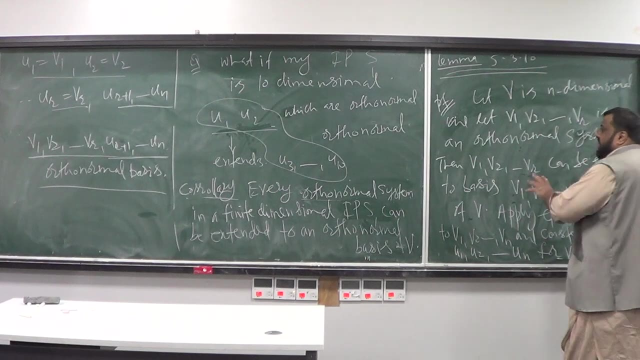 I am doing a lot of waving of hands because I am assuming that you know the linear algebra, the first linear algebra course, very well and you know the Gram-Schmidt process, so I am not spending too much time on it actually. ok, so what is the conclusion? 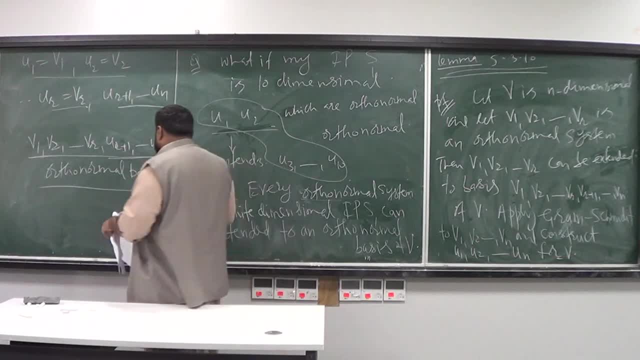 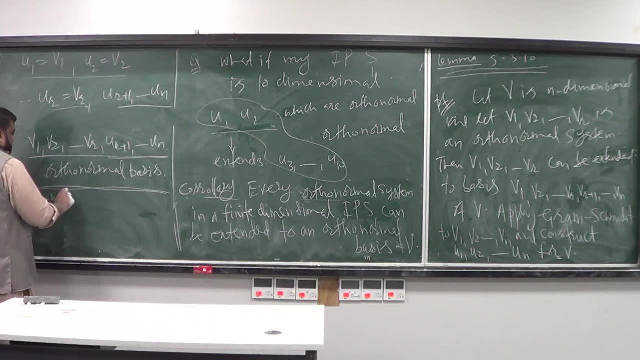 in this, in this, this section, we we defined what is orthonormal system. ok, what do you mean by orthonormal system? we did some examples of it. we showed that orthonormal systems, orthonormal systems are linearly independent, are linearly independent. and then 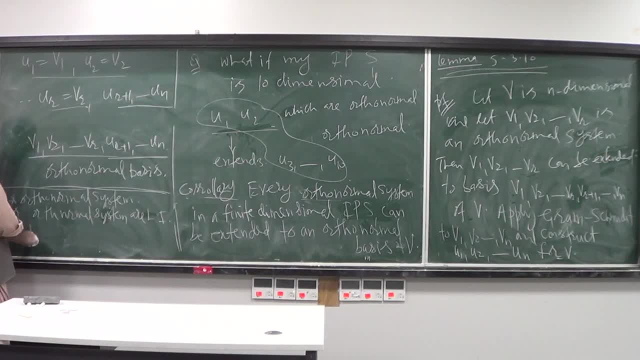 we showed that the key result is every finite dimensional vector space, inner product space. so if you have a finite dimensional inner product space, that inner product space has an orthonormal, orthonormal basis. and then, finally, we showed that if you take some number of orthonormal basis, 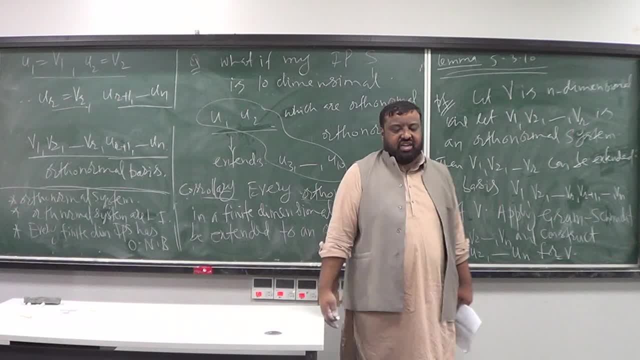 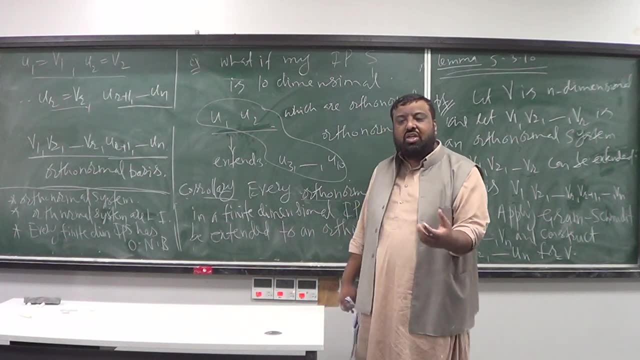 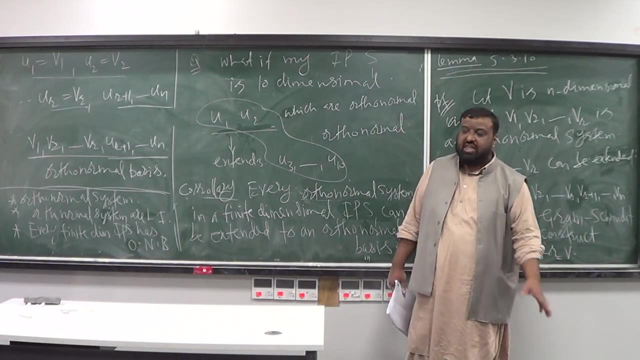 vectors in an in a finite dimensional inner product space, you can some add, some cleverly, add some more vectors into those orthonormal vectors and create an orthonormal basis for the entire vector space actually. ok, so this is a set of discussions that we have. 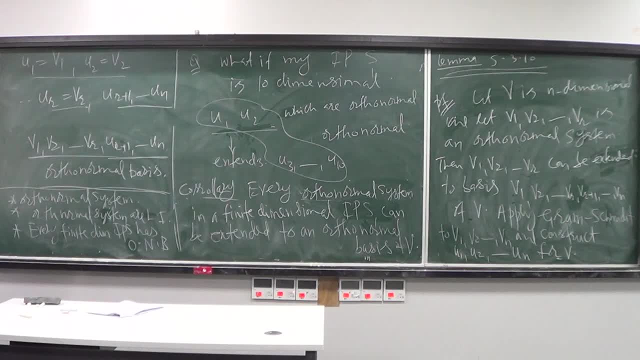 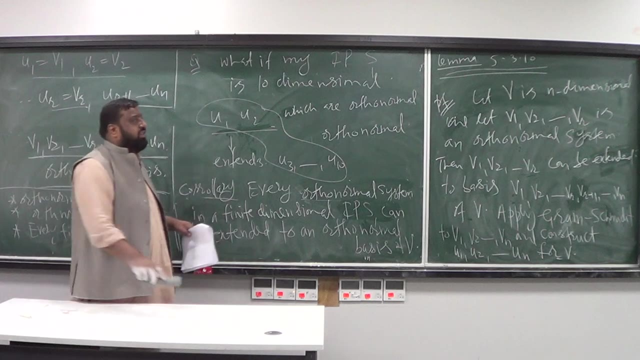 done so far, and now I would like to move to the next session, the next section, and in this section I am going to get into the details of every single thing. ok, so I keep on saying to everyone: really the over 90% of mathematics is linear algebra. 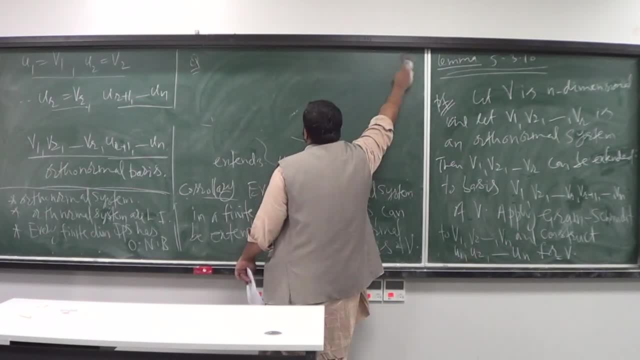 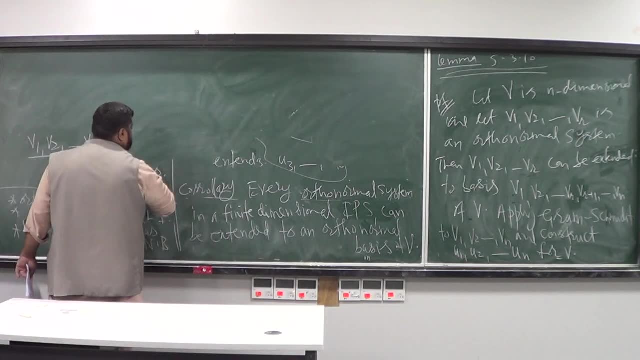 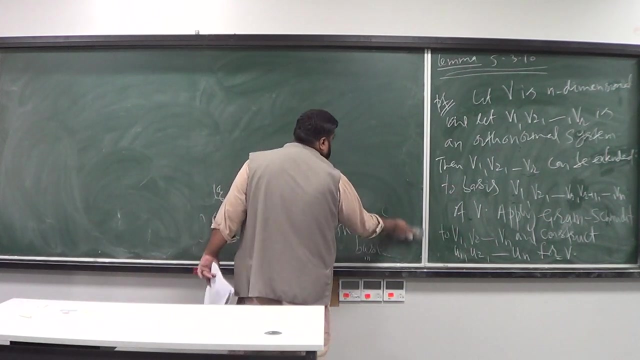 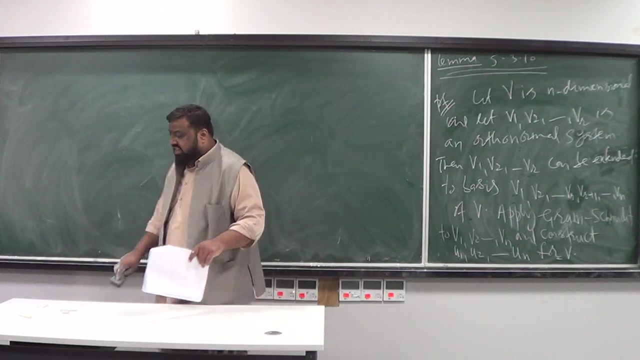 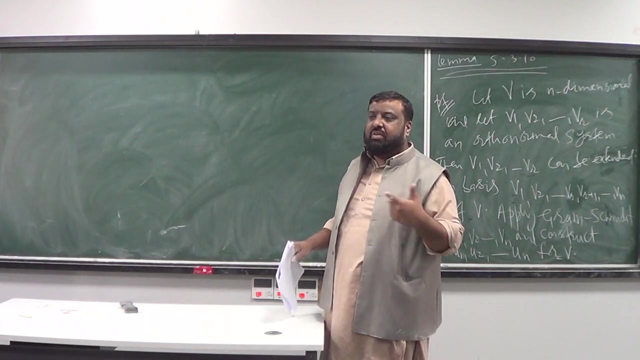 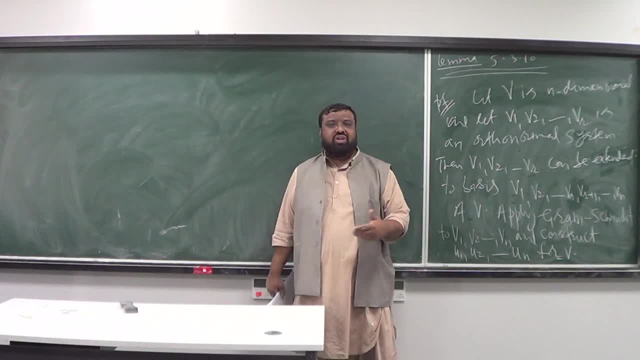 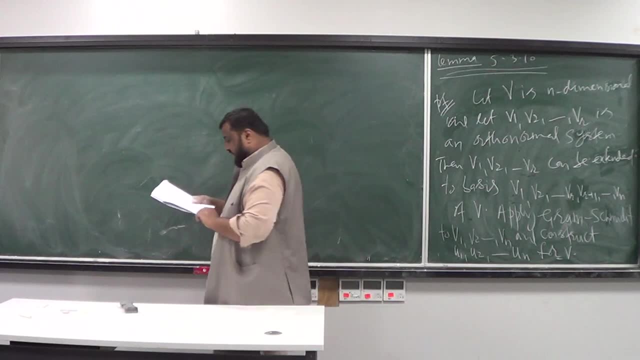 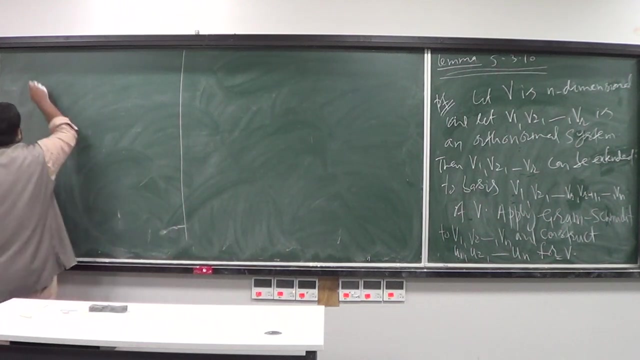 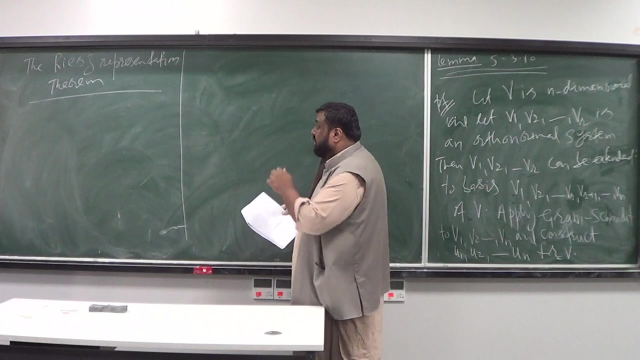 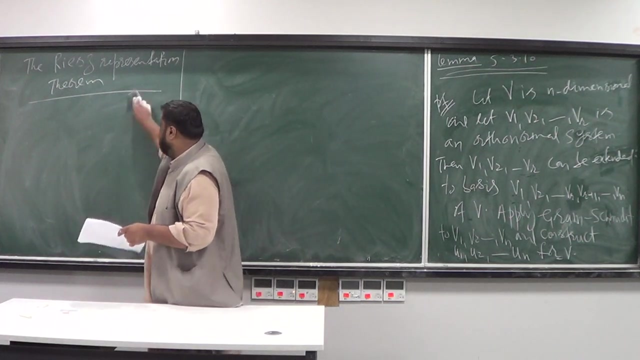 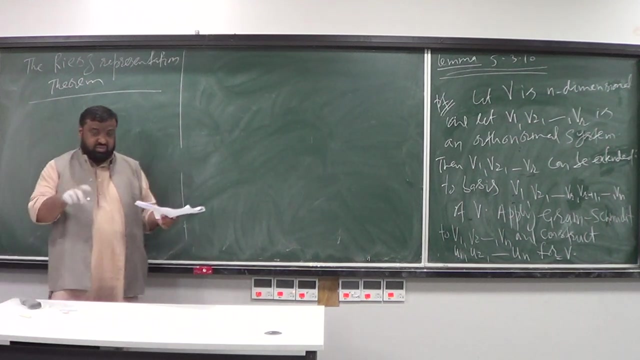 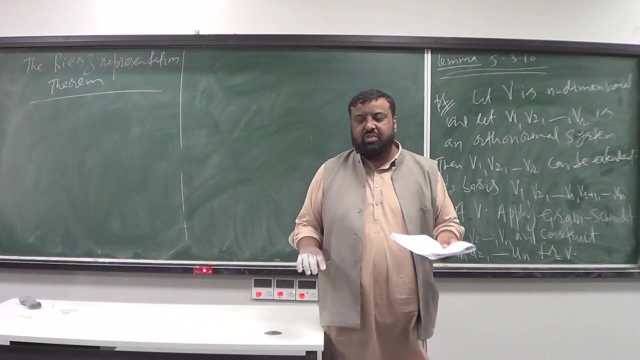 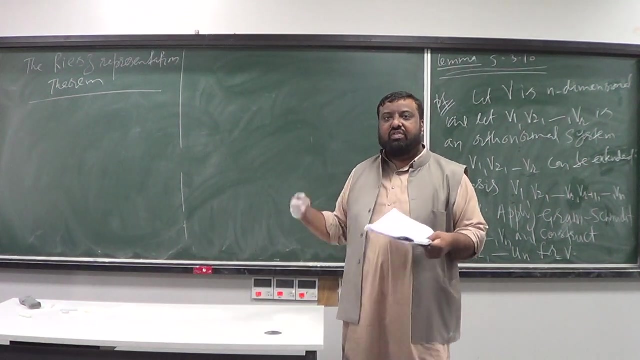 and, and, and, and, and, and, and, an, and and and an. so you will see that if you have an inner product space with an orthonormal basis, so the most of the time now on, whenever we are going to discuss an inner product space, we will always consider an orthonormal basis of it, because we proved, just proved, or we 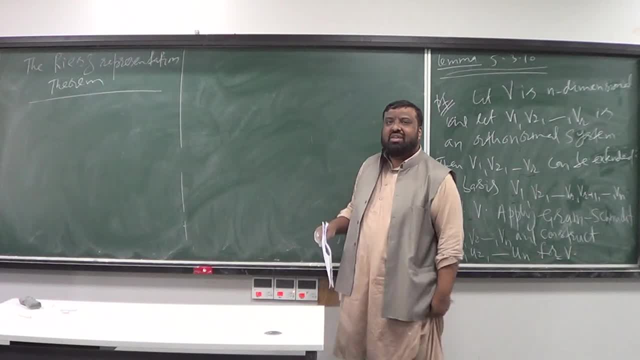 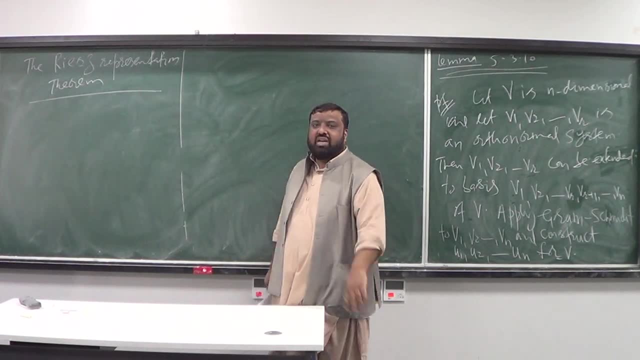 just saw that every single you know, inner product space or finite dimension, inner product space- always have an orthonormal basis. so we are going to make our life easier and always consider an orthonormal basis. So lets start with the orthonormal basis. 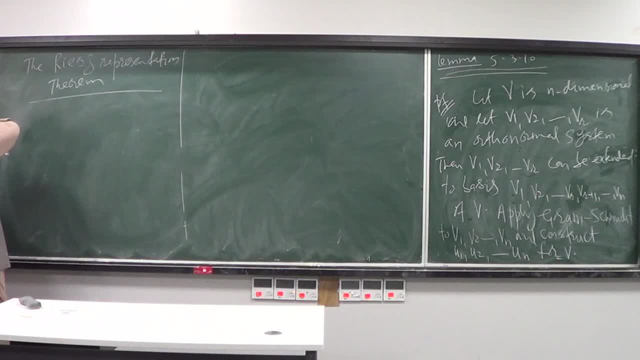 This is what you call a new class of linear transformation, called the linear functional structure. linear functional, linear functional. ok. so what is the linear function? here is the definition. So what is the linear function? Here is the definition. So let V be a vector space over a field F. ok, then a linear transformation. ok, then a linear. 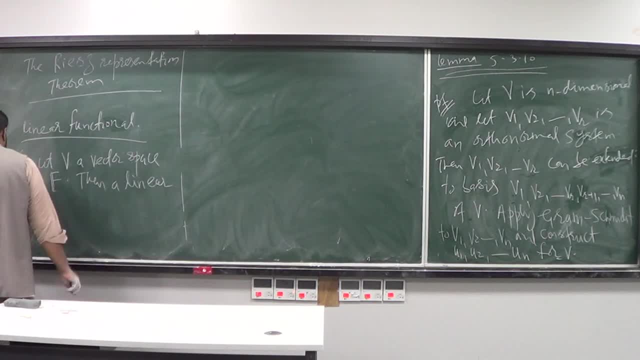 transformation, ok. So what is the linear function? Here is the definition. So what is the linear function? Here is the definition. We call any linear transformation F. ok, or maybe phi, you know any symbol you like- from the vector space. This is important. 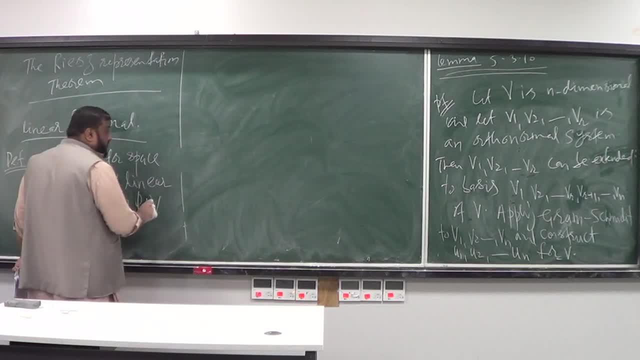 From the vector space, not to another vector space. Okay, From the vector space, not to another vector space. What is V? V is the new state, but to its field and, by the way, we know that every field is a vector space as well. 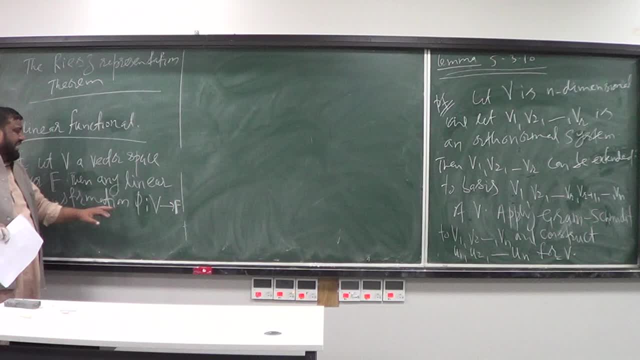 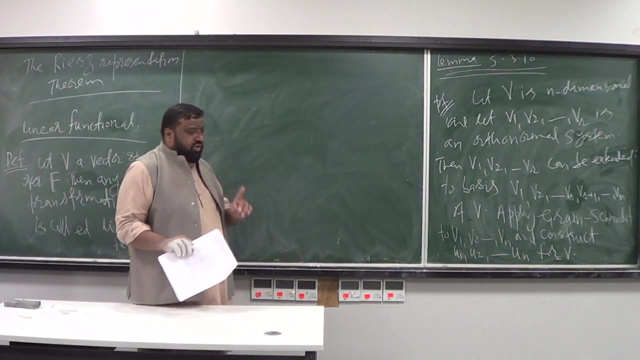 so a linear transformation from a vector space to its field. you call such linear transformation as a linear function. you call that linear transformation as linear functional. you call that linear transformation as a linear function. so what's a linear functional? linear functional is a linear transformation from the vector space. 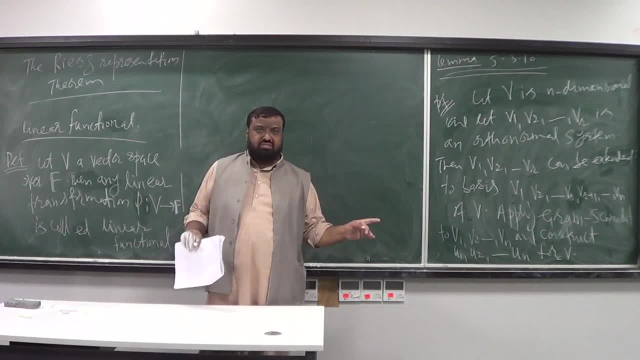 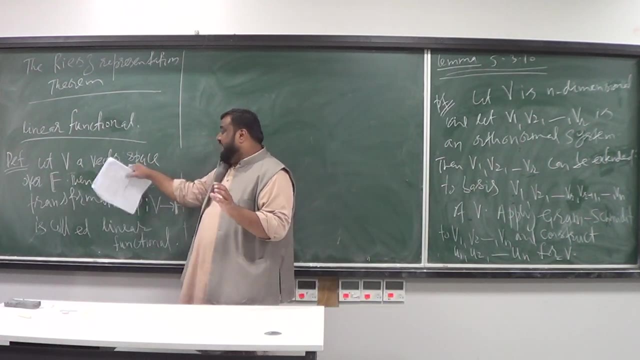 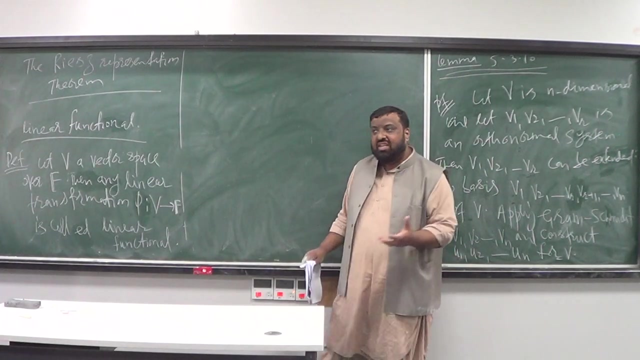 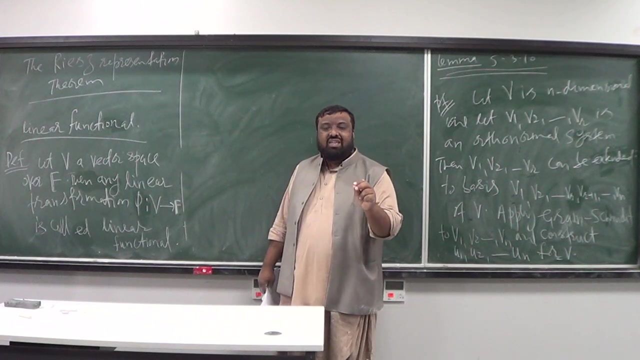 whatever your vector space is to its field. this is what and what we will do basically in this theorem or in this section, is that if you consider the vector space as an inner product space with an orthonormal basis, then any linear functional, any linear functional, can be written. 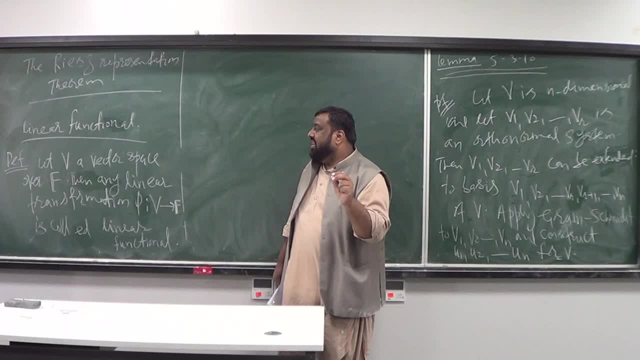 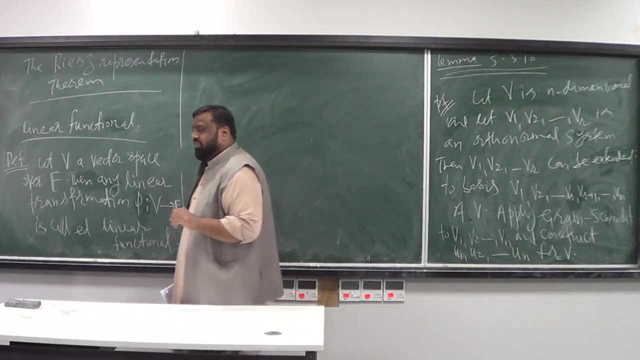 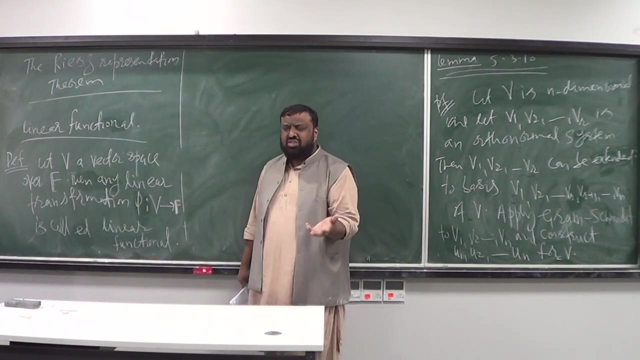 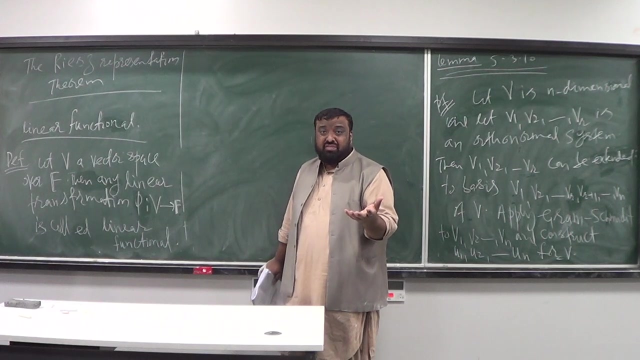 in a very interesting way, in a very interesting manner in the terms of the inner product. so it kind of classifies all kind of linear functionals. so all linear functionals on a finite dimensional inner product space, and it is also true in infinite dimension, can be written in a very simple form actually. 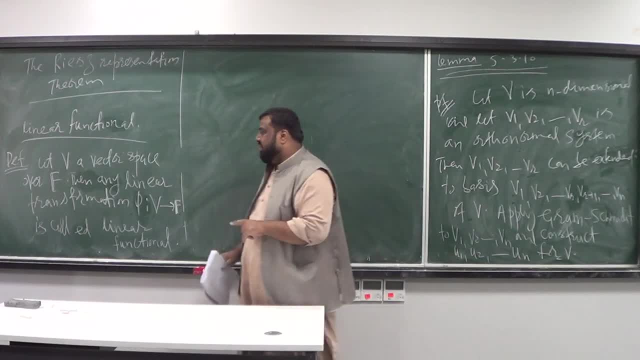 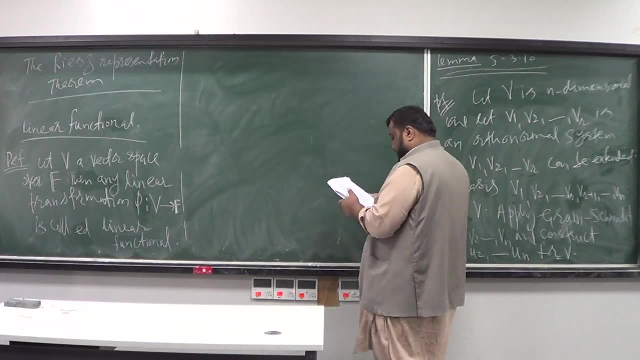 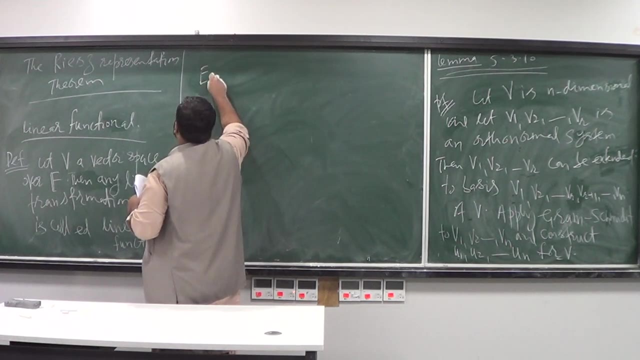 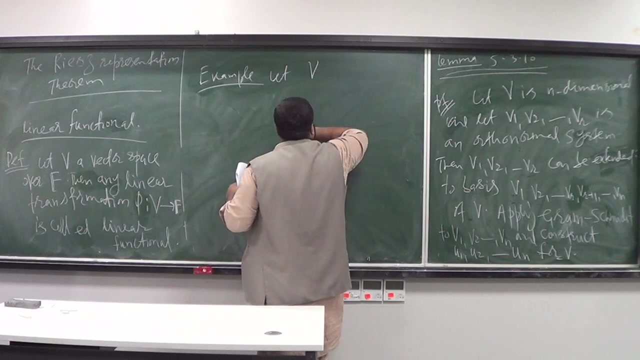 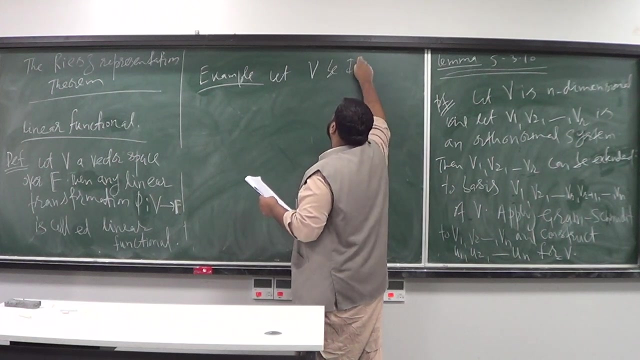 in a very particular form in the terms of the inner product. so we are going to get into that. we are going to do some examples of linear functional actually. so, for example, the first example is: first example is that you take any inner product space, let V be any inner product space over F. 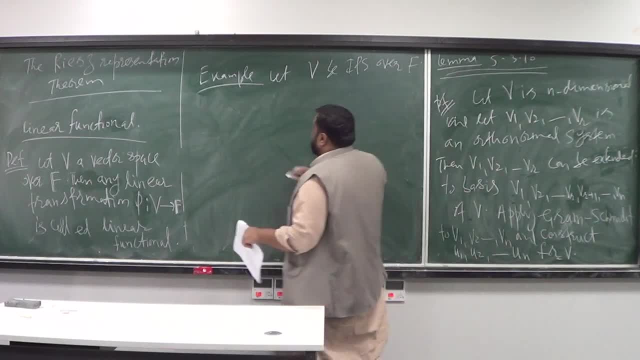 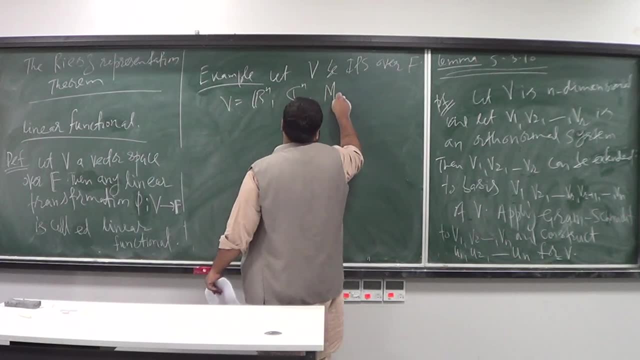 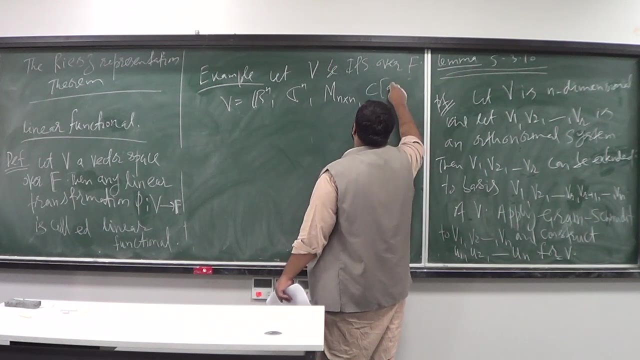 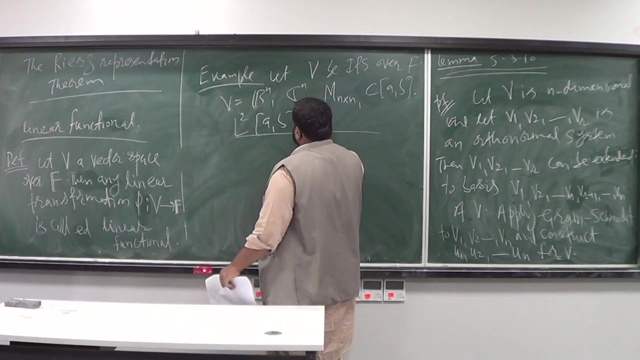 so it could be. so this means that this V can be Rn, it could be Cn, it could be the space of all matrices, it could be C01 or Cab, it could be L2ab, it could be anything. so we discussed all such examples and many such examples. 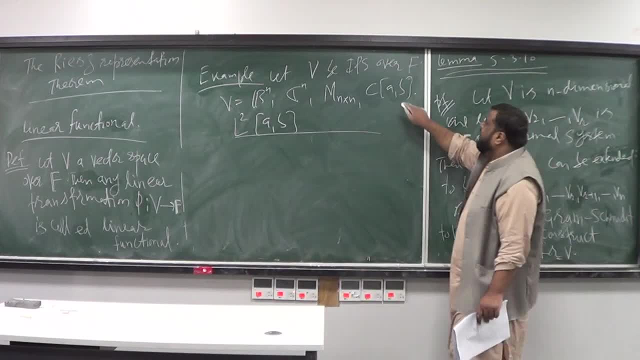 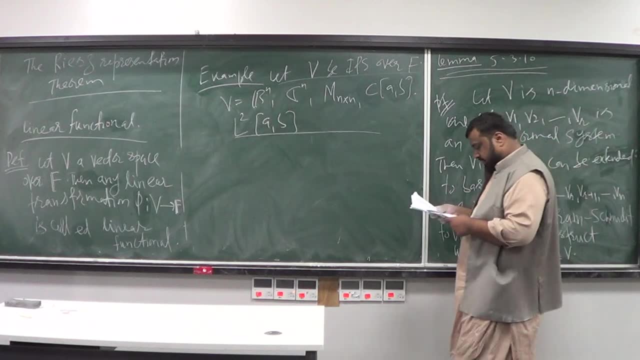 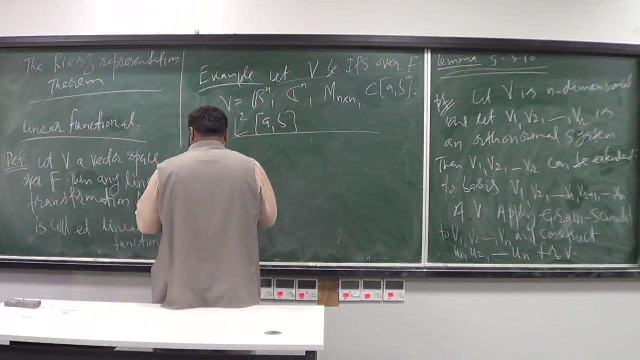 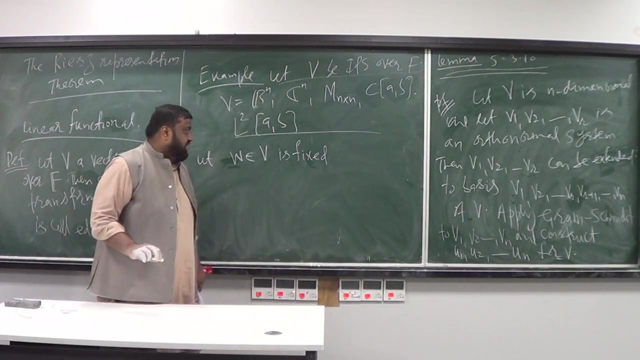 in the chapter of inner product space. so imagine you have any inner product space, any inner product space. then in that inner product space imagine you take a fixed W, so a vector W, whatever. let W in V is a fixed element, then corresponding to this fixed element, W. 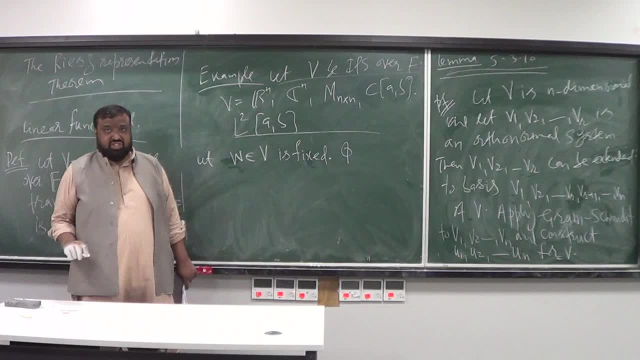 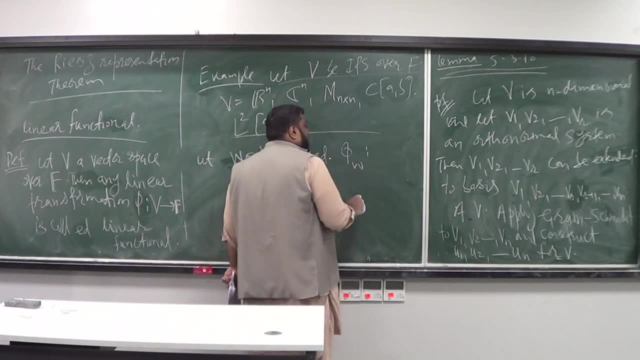 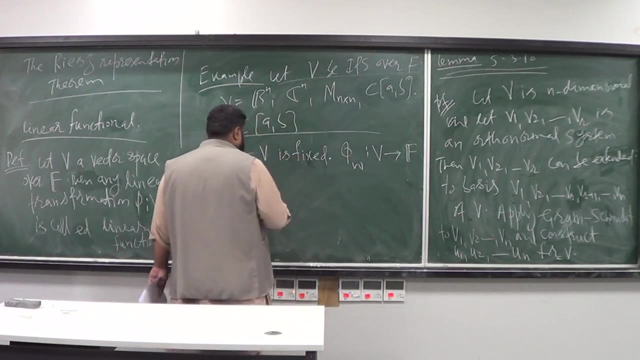 you can define a linear functional. let's give this linear functional a name: W, phi W. so phi W is going to be a map from V into what you call feed F, and the definition of the phi W operated onto V is going to be what just compute the inner product of V. 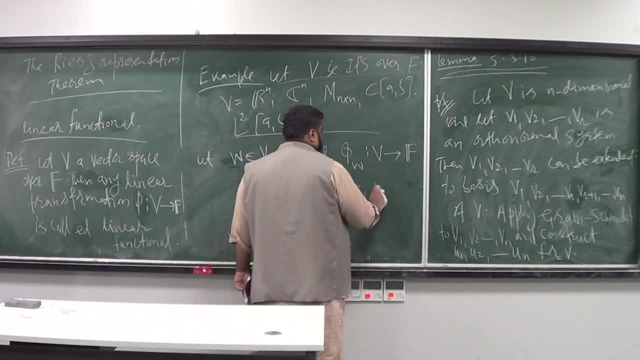 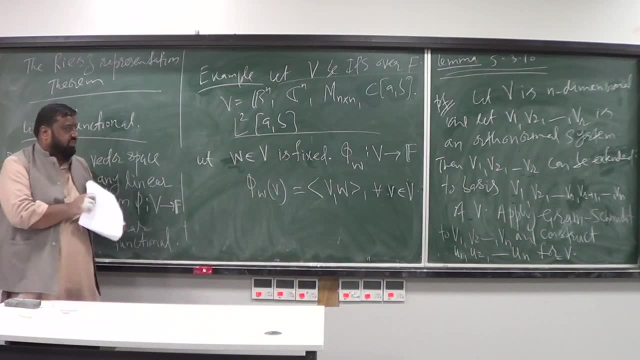 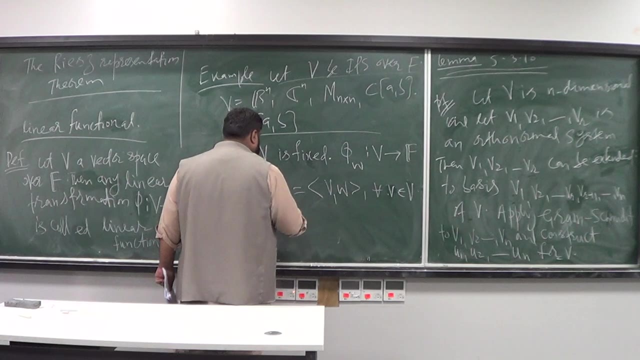 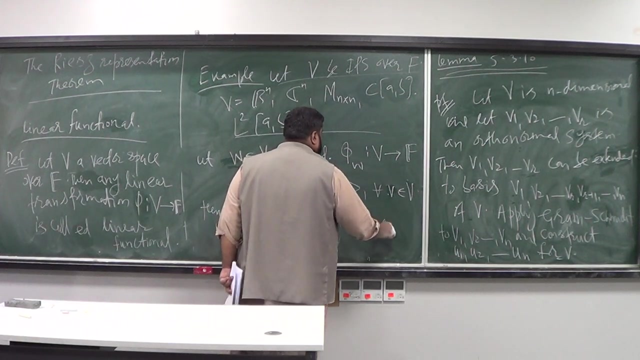 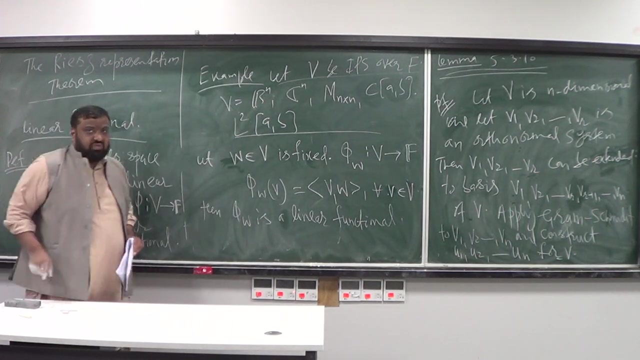 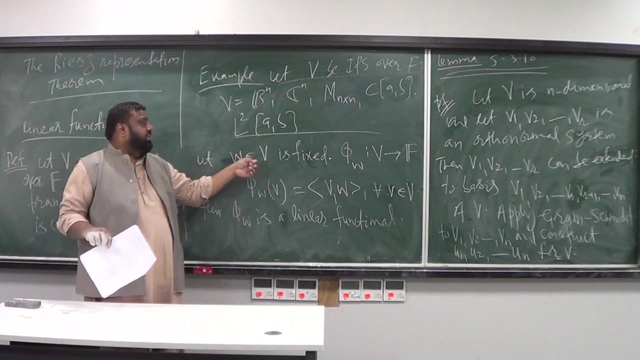 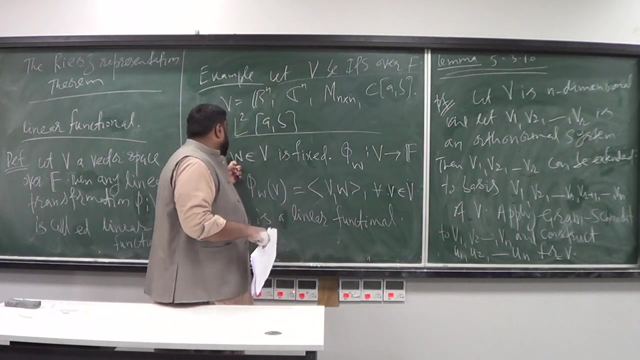 with this fixed element W for all V in V. ok, for all V in V, then this phi W is a linear functional. ok. so this is a very interesting observation: to every element in element in the inner product space you can always find a linear transformation, so corresponding to every element in vector space. 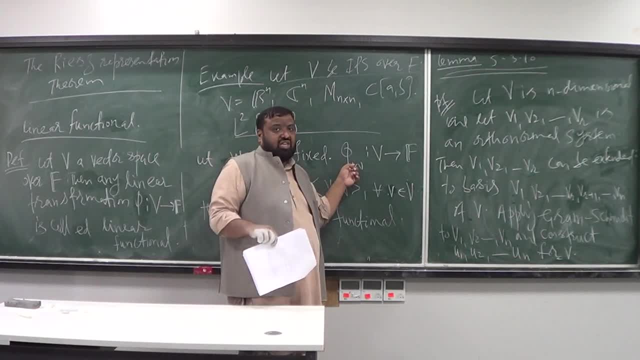 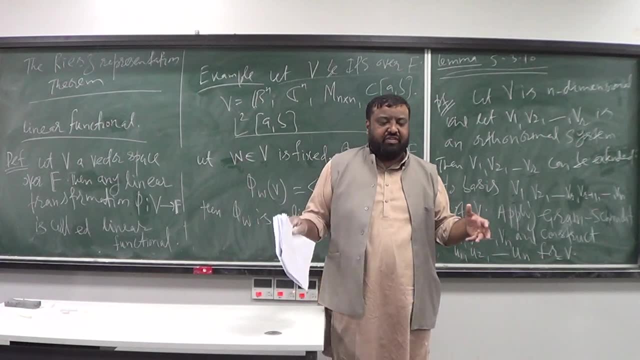 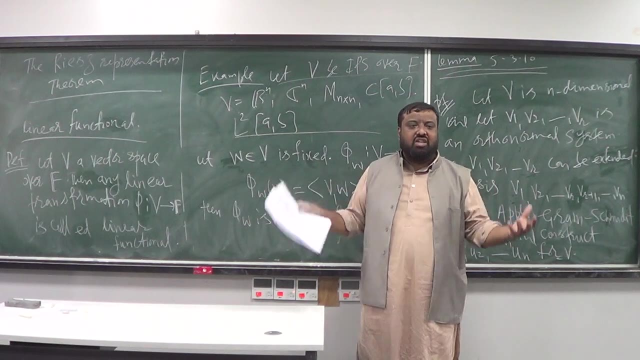 you can always find what you call a linear functional. ok, and then when we will move ahead, we will see actually that the collection of all such linear functional. so for every element in inner product space you have a linear functional. so the collection of all such linear functional. 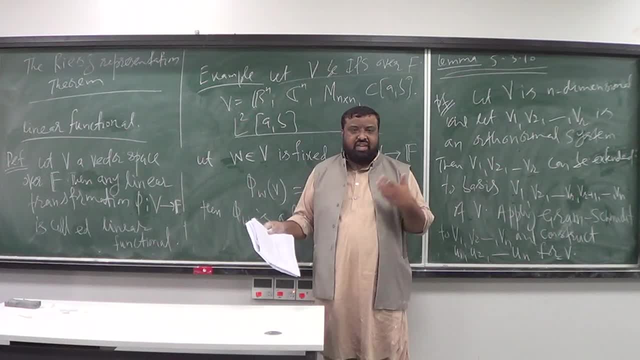 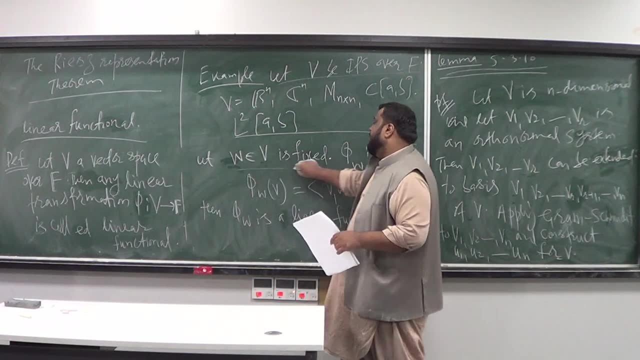 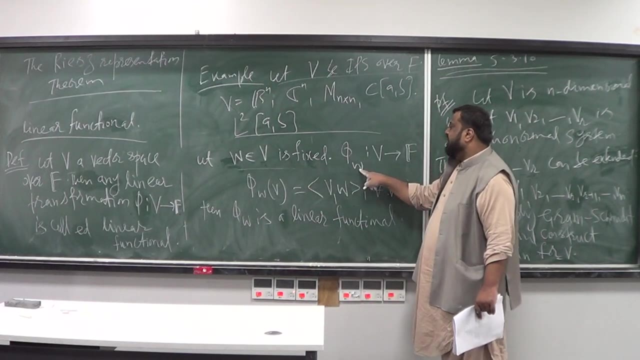 also becomes a vector space, and you call that vector space as a dual space actually. so I am not going to get into that, but you know for now what I did: take W and using this fixed W, I can define a map that depends on W, such that: 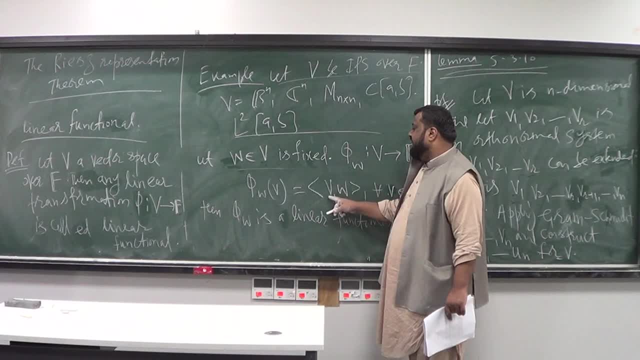 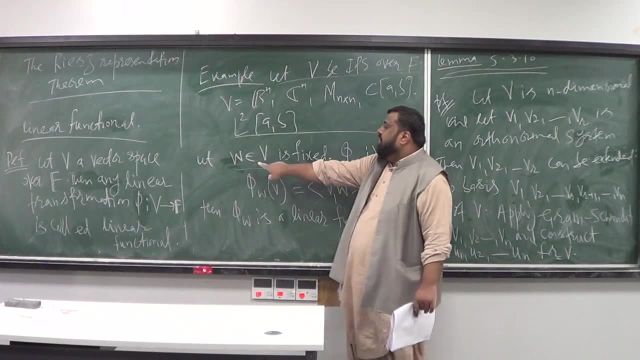 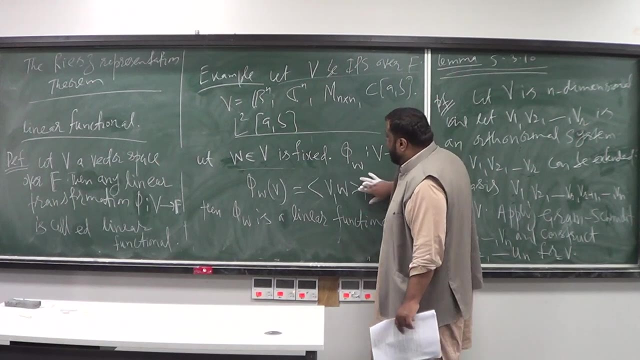 that phi W, operated onto any V, is going to take the inner product of the V with this fixed element, W. ok, so in other words, take W and take the inner product of W with every single element in the V. that map is going to be a linear, functional. 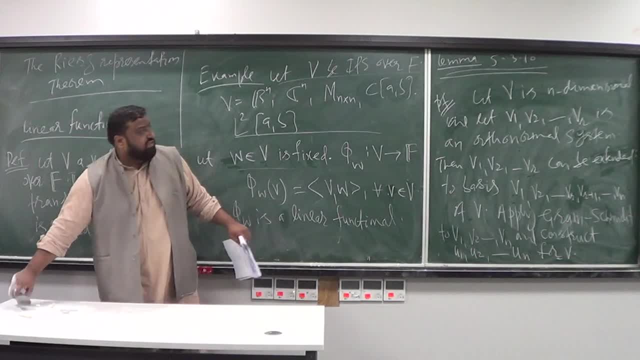 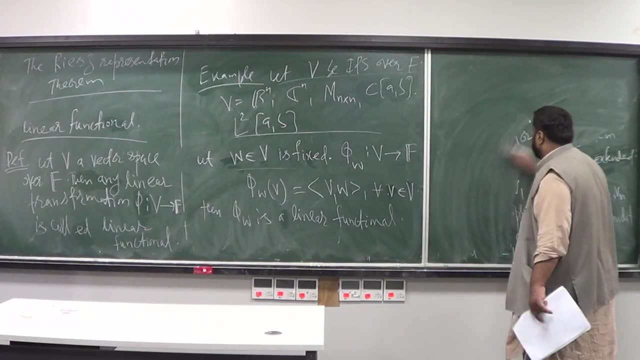 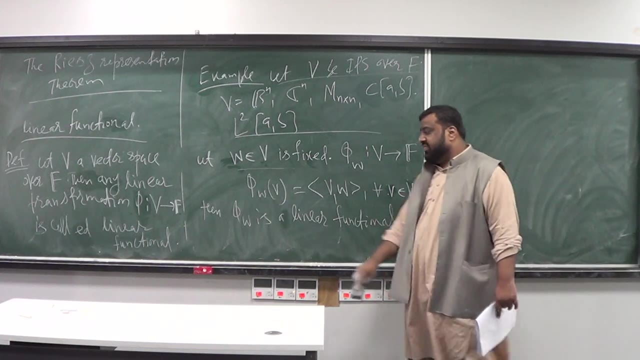 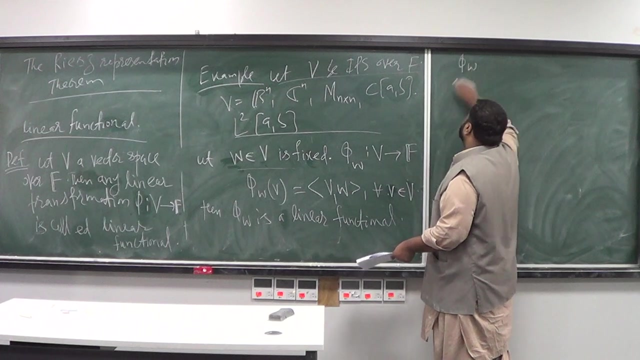 so why it is going to be a linear functional, it is not difficult to say. and then we are going to get into some concrete way of it, concrete situations actually, ok. so so to show that this is a linear transformation, I need to apply it onto, say a: 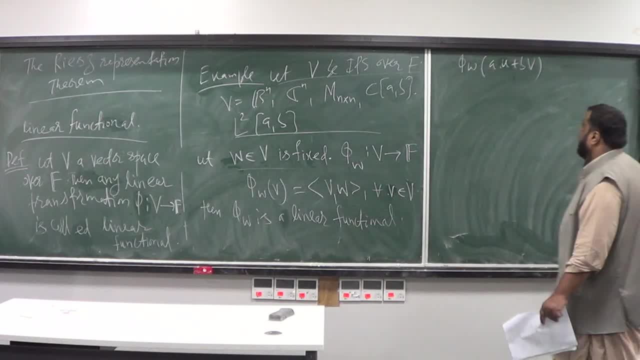 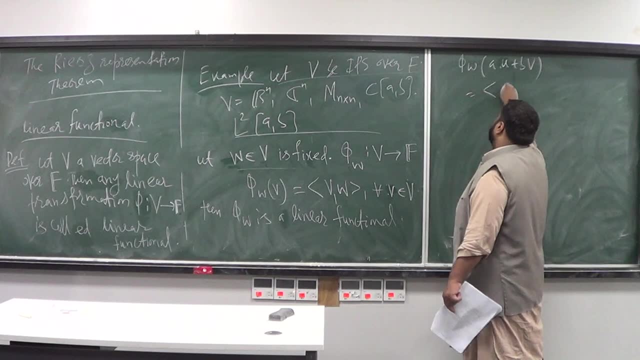 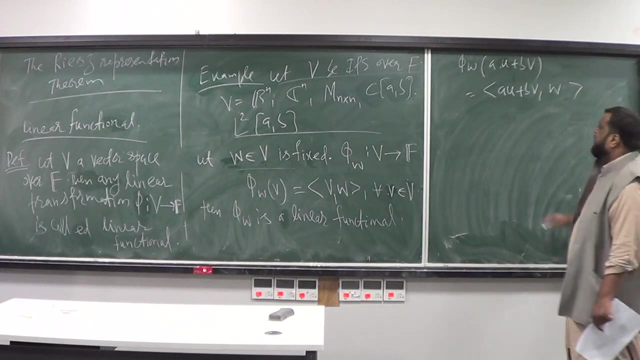 some vector, AU plus BV. ok, where A and B are scalars and U and V are vectors. in the the inner product space, V. by definition, I can write this as AU plus BV and its inner product with fixed W. then by properties of inner product, I can write this as: 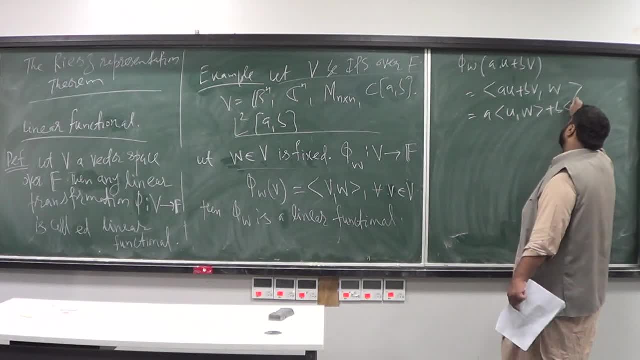 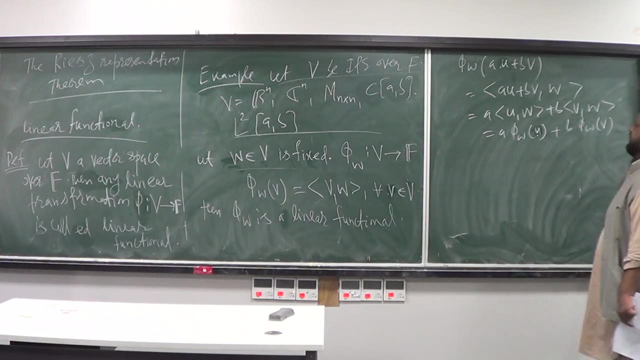 AUW plus BV VW, and hence this will become A phi W of V plus phi W of U plus B phi W of U by definition, and obviously this shows that this map phi W preserves the addition and the scalar multiplication of the inner product space, or the vector space actually, and hence 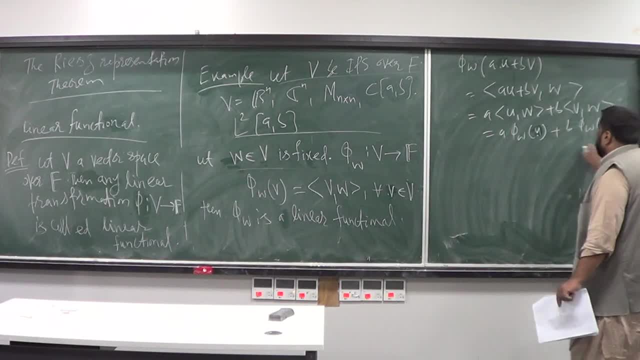 this is a linear transformation, ok, so let's take- let's take this V in what do you call in some concrete situations. actually, ok, let's take this V and take it into a concrete situation. for example, let's consider this, this linear functional here, actually in CAB. 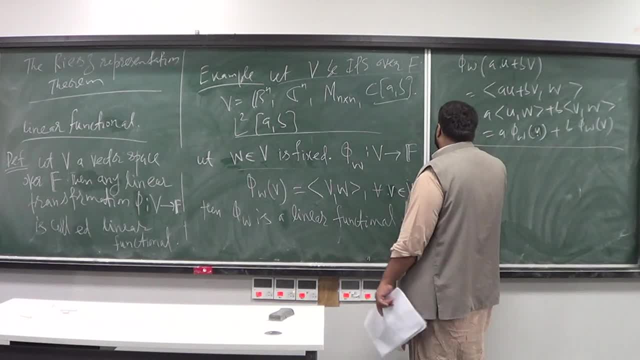 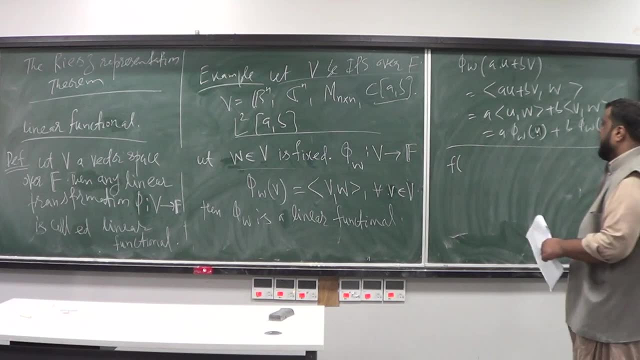 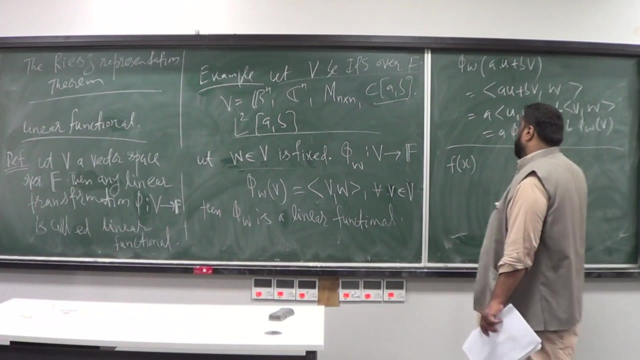 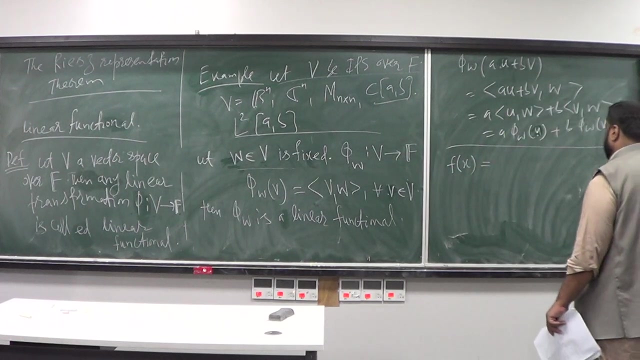 so, so. so let's take, for example, let's take, say, for example, f of x to be. let's take f of x to be, for example, where x is in the interval A to B to be some function. ok, some function. so I don't know, let's call it x actually. 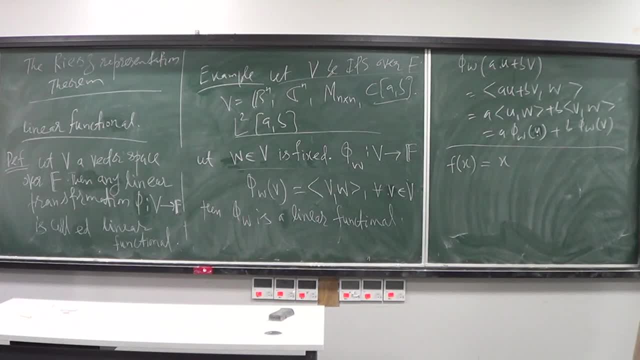 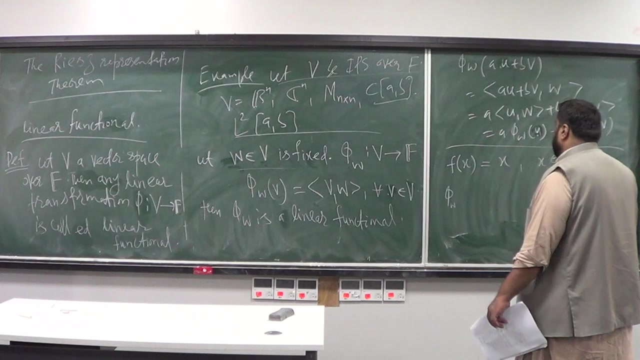 ok, so let's call it x where x is in. what do you call AB? so it's a polynomial x. ok, x is in the interval A to B. ok, so what would be the inner product? inner product corresponding to this: f for phi for W. so I must write in: 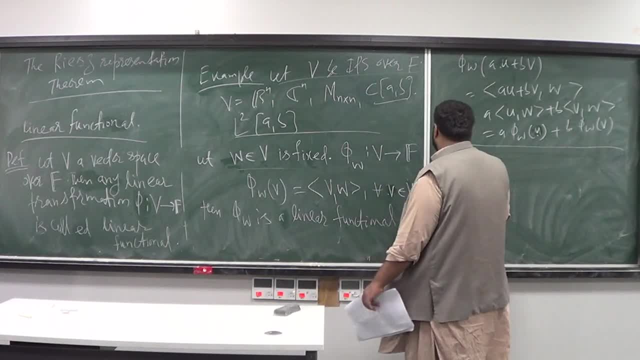 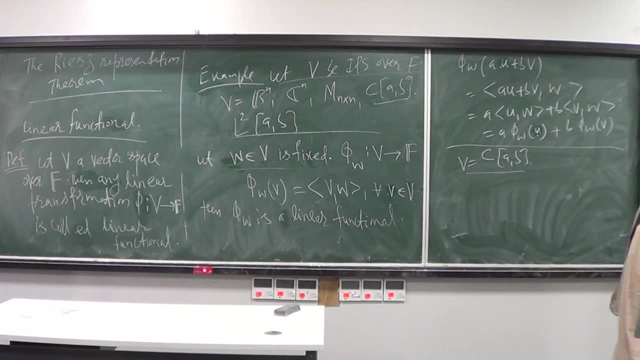 more explicitly that I am considering V to be CAB, ok, space of all continuous functions defined on an interval a to b, then we know that on this interval we have this inner product, which is simply the product of af, of x, g, of x, dx. in other words, multiply and take their integral, because f and g are continuous, their product is continuous and hence, you know, for continuous functions the integral makes sense, so inner product makes sense. you can prove that this is inner product. 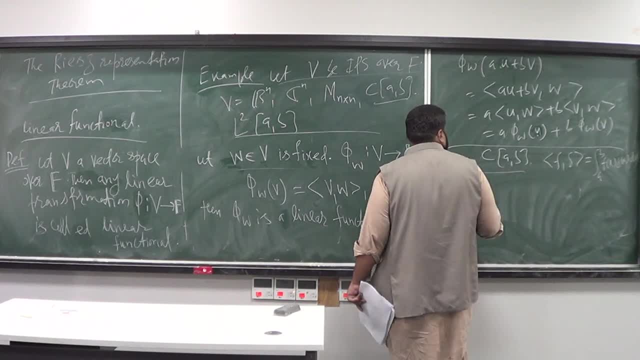 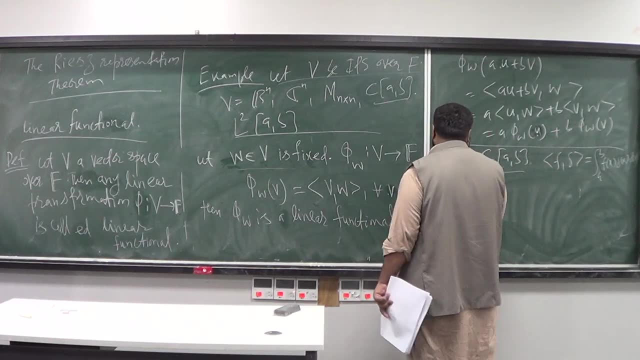 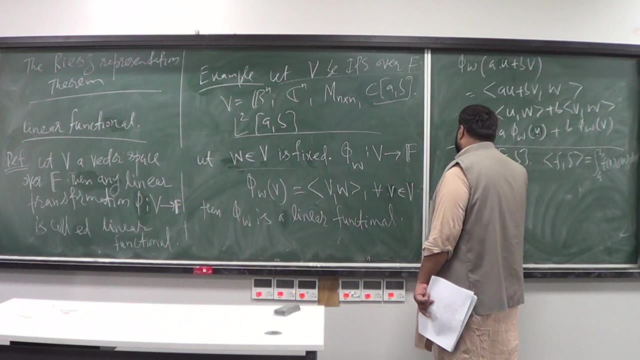 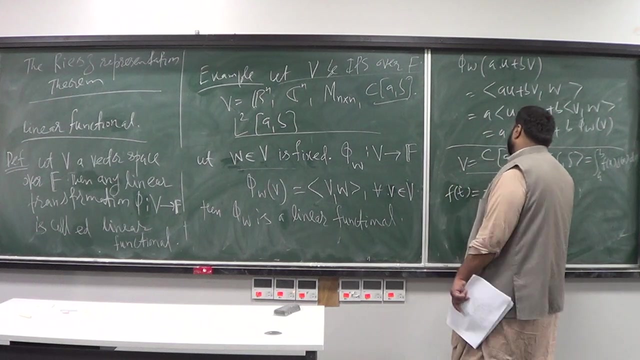 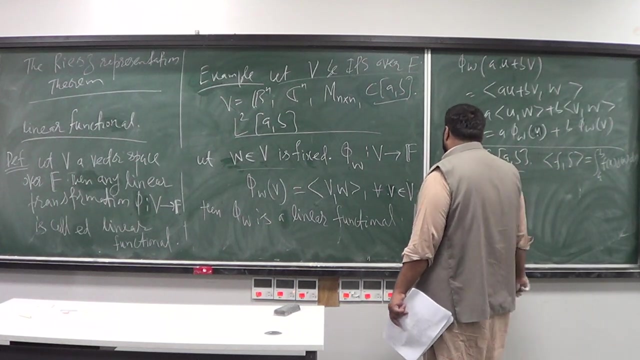 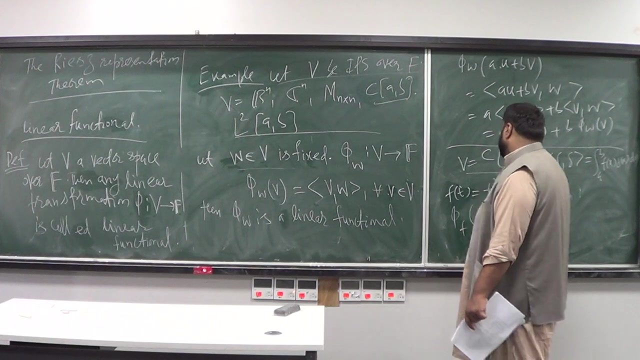 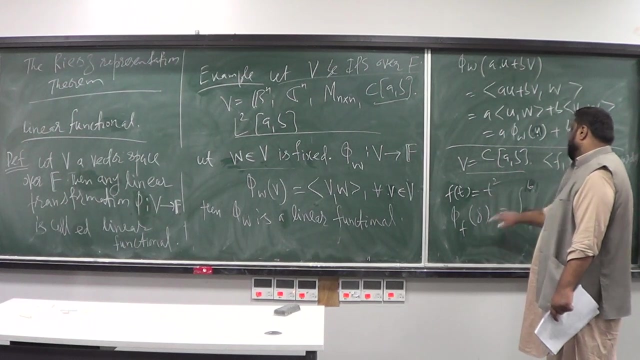 and now I want to take for example a particular function. okay, so, for example, I want to take: say f of t, equal to f of t, equal to what do you call. take any function, say t, maybe t square, something like that. okay, then an example of linear functional corresponding to this function: t square f, operated onto some g is going to be what that? take the integral from a to b and multiply the f and take the inner product of f with g, which means that take f of x and take g of x, dx. 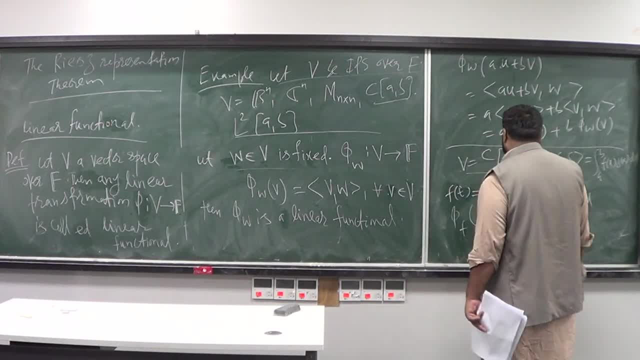 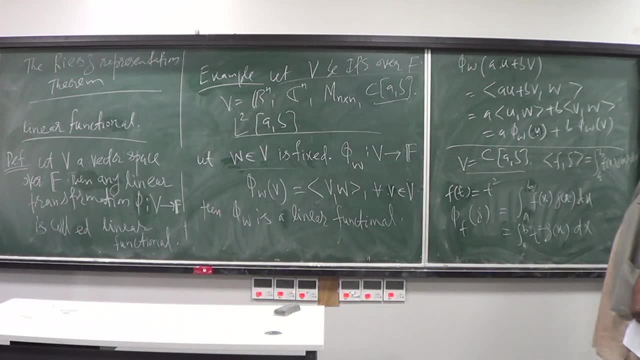 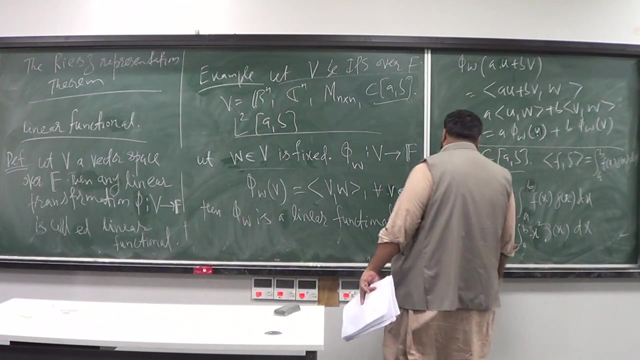 a to b, okay, and you are going to have t square g of x, dx, actually x square g of x. So this is what is going to be. so this is a linear, functional okay. and the interesting case also, that would be that, for example, when you take f of x, equal to 1, actually, 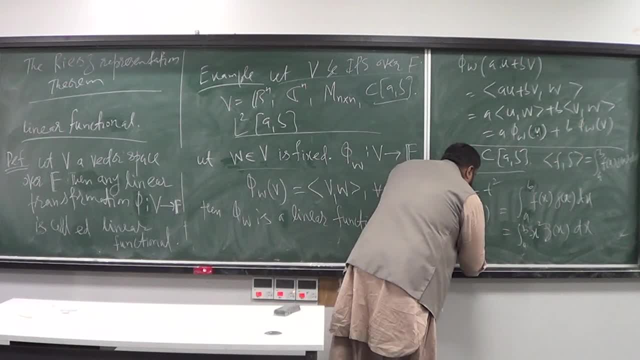 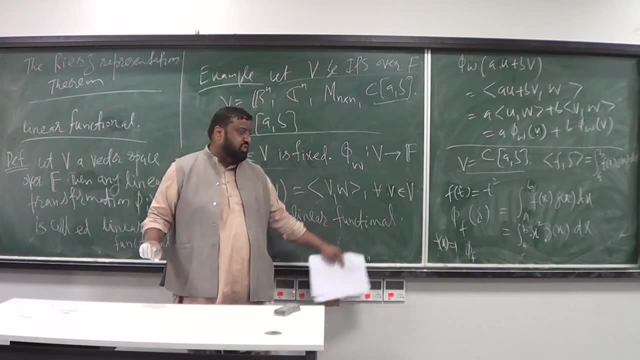 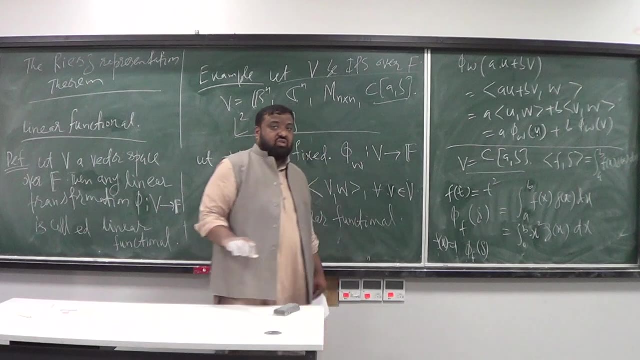 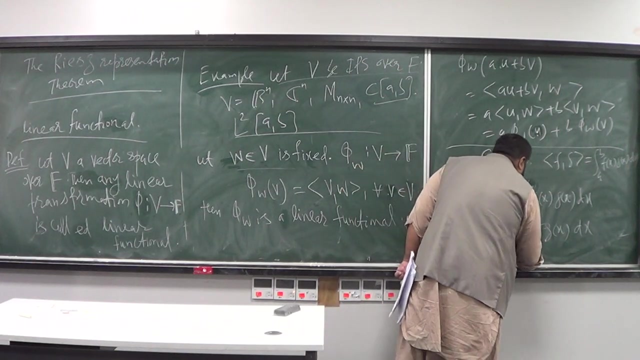 So what would be? f of x? So what would be, what is the linear function that we can approach, the linear transformation that is corresponding linear functional, that is corresponding to this F, So, by definition, by F of g, So, by definition, this is going to be equal to the integral from a to b of g, of x, dx.